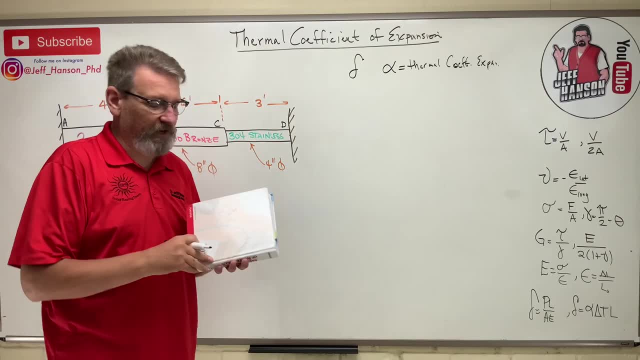 it's a look them up. So if you have your material table, you flip that open to the very back page. we'll see what it is, And that is the thermal coefficient of expansion. We're very familiar with this table, aren't we? And you just read across here. let's see. 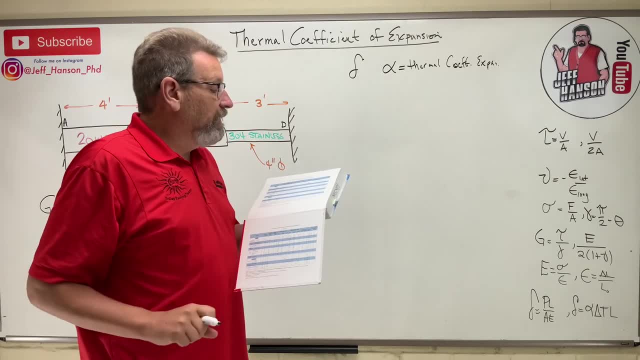 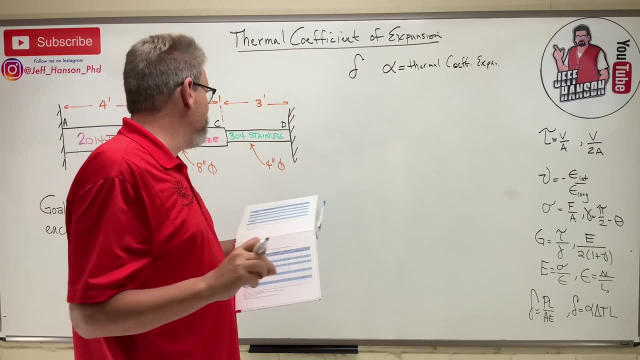 where is it? Oh, it's the very last column and it tells you the thermal coefficient of expansion, and it's a very small number. For instance, for aluminum 2014 T6,. hey, that's one of the ones. 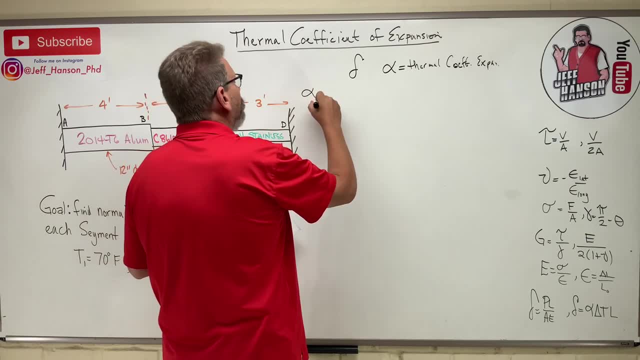 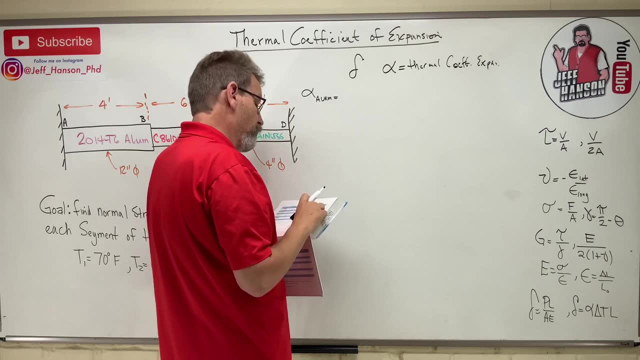 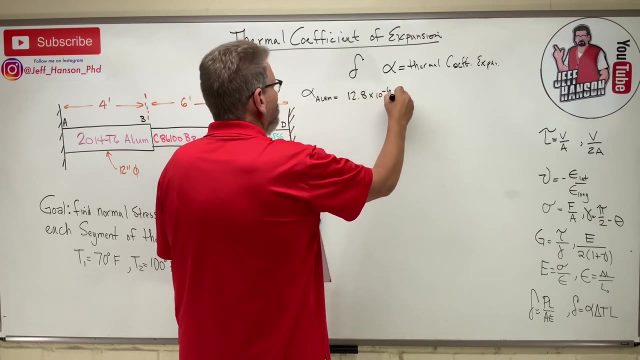 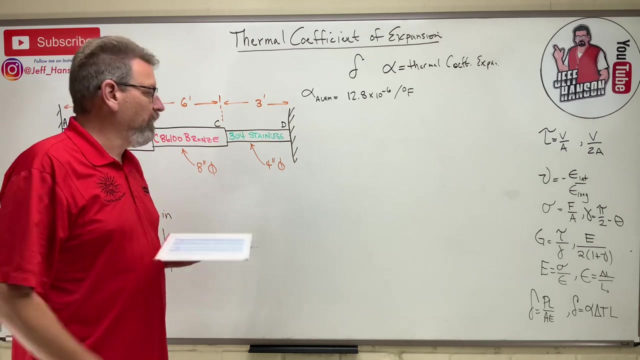 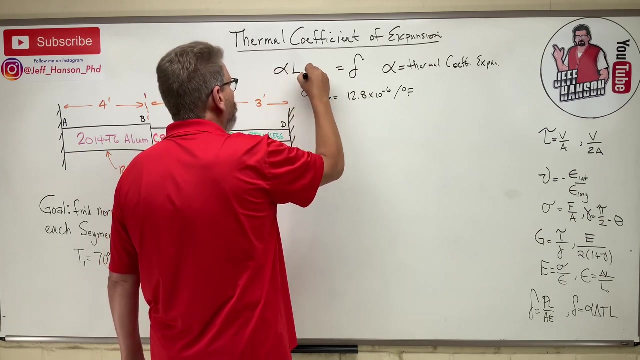 we're working on today. Alpha for aluminum 2014 T6 is 12.8, times 10 to the minus 6 per degree F. Isn't that a weird unit per degree F? Well, we have a new equation for this delta here, and our equation is this: alpha L, delta T- okay, 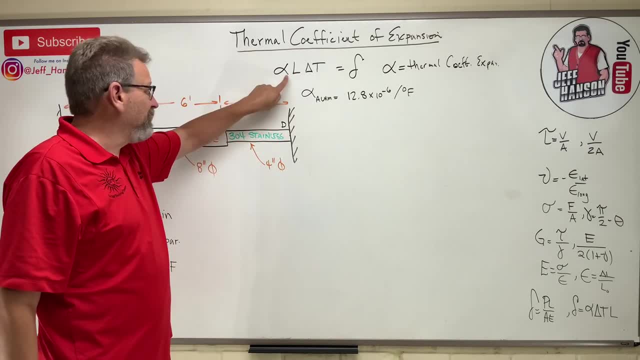 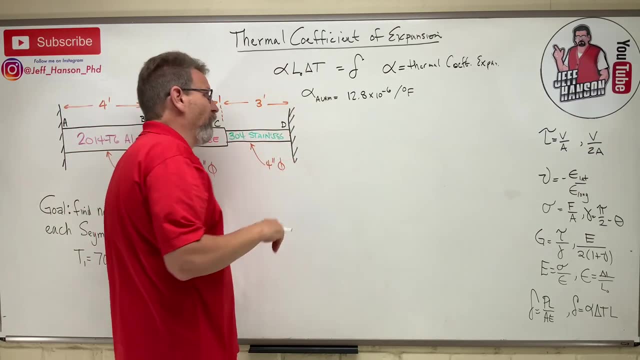 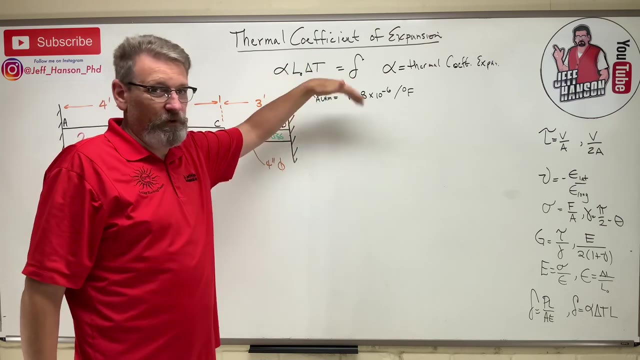 So alpha is the thermal coefficient of expansion, L is just the original length of the material. we can put L, O for original length, right. And then delta T is the change in temperature. Now that's going to be in Fahrenheit or Celsius when you're talking about SI units, or 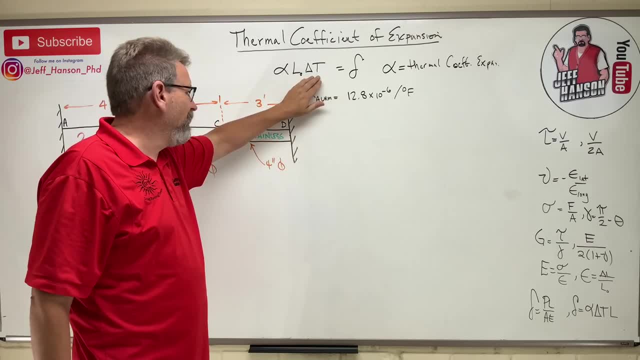 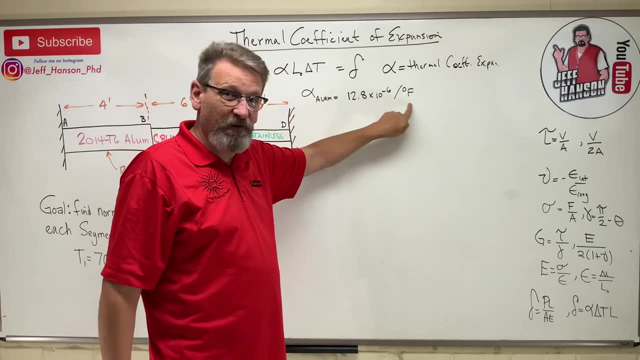 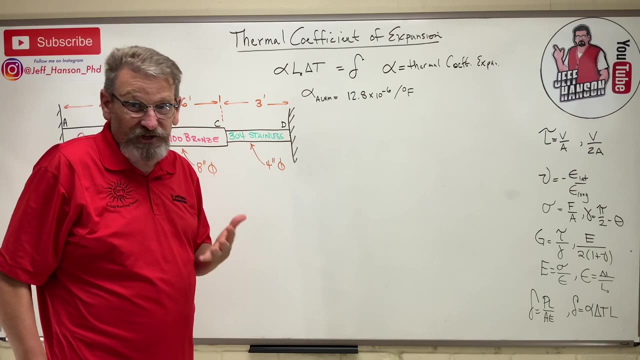 US customary units. okay. So if that's in, if that is in degrees Fahrenheit, and this guy over here is in per degree Fahrenheit, whoop, whoop, those units cancel out and they're going to leave you with just a length. right, And that's what the delta is. it's a change in length. so 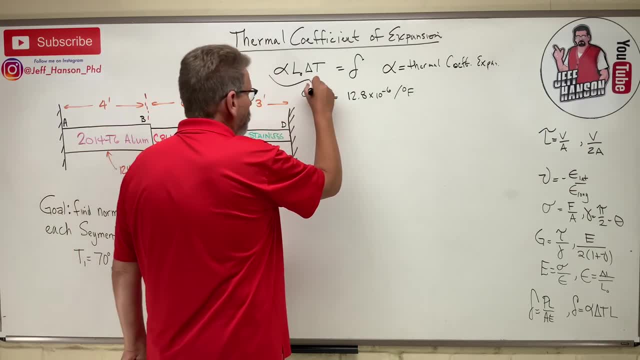 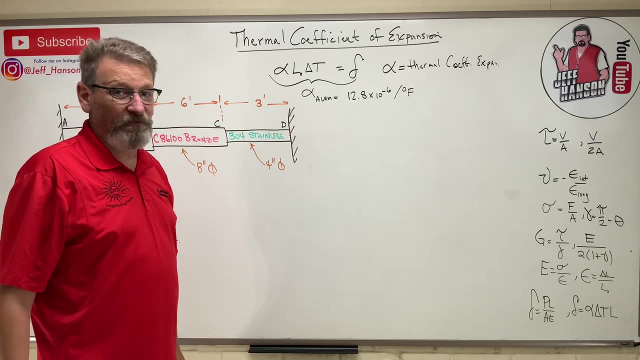 that makes sense. So this is the new equation of the day, and I have taken the liberty, bam, to add it to our list of equations. It's getting kind of long of things that we need to know, isn't it Okay, so for this. 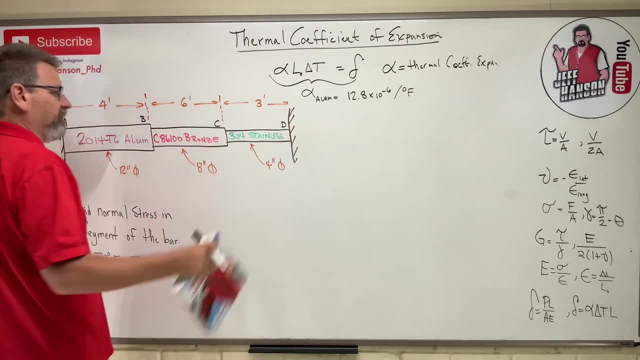 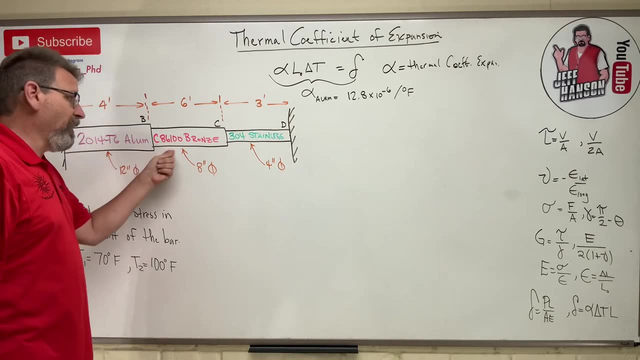 little problem. we have two walls- wall here, wall there- and we've got this three-step bar in between, and it's made out of three different materials: aluminum, bronze and stainless steel. Excuse me the diameters that's. 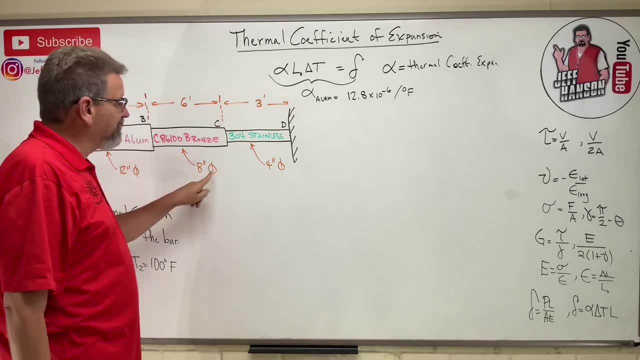 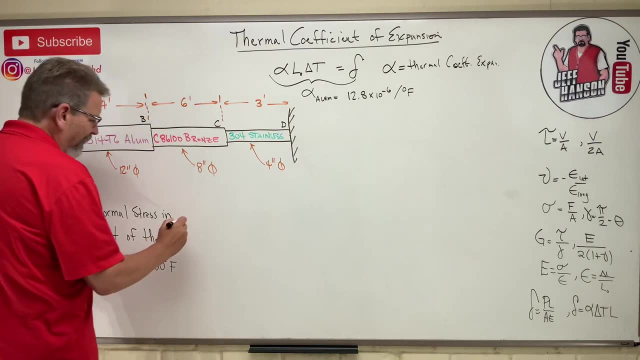 that's a symbol for diameter, are 12 inches here, 8 inches there, 4 inches there and of course, the length's up here. So they want us to find the normal stress. normal stress, What is normal stress? Oh yeah, that's. that's sigma stress, isn't it? So that's a force over area, isn't it? 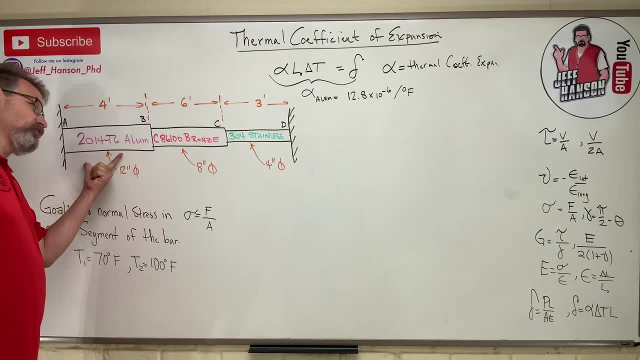 So they want to find that for each segment of the bar. So what's the stress here? What's the stress there? What's the stress there? The temperature goes from 70 to 100, okay, So the temperature is going up. 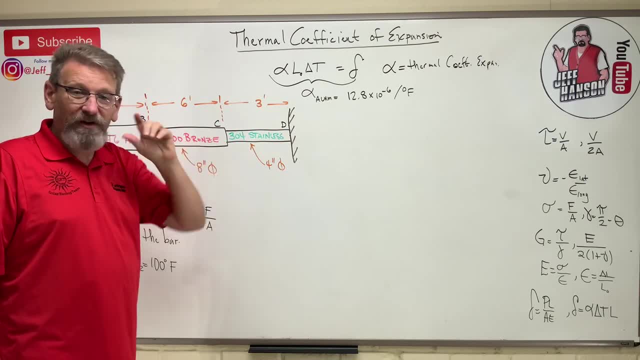 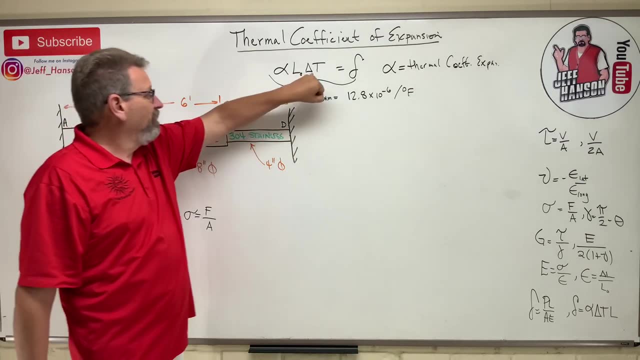 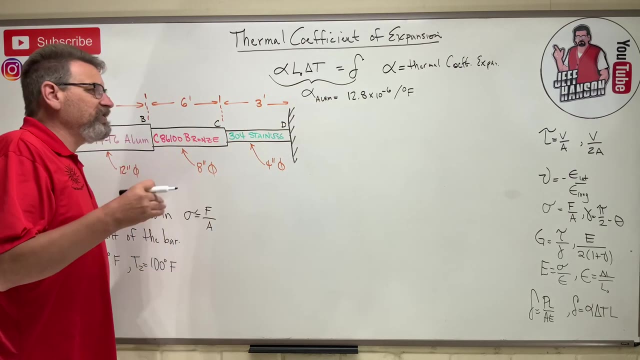 What happens if the temperature goes down? Well, instead of the bar getting longer, the bar gets shorter. right? If delta T is negative, then this becomes negative, and so your delta for the growth is negative. all right, So here's how you solve this problem. okay, Number one, let's. well, I got. 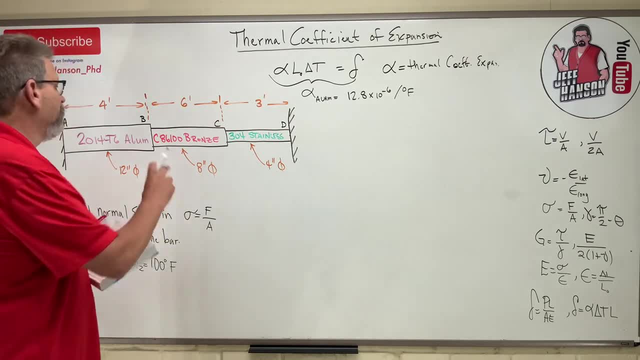 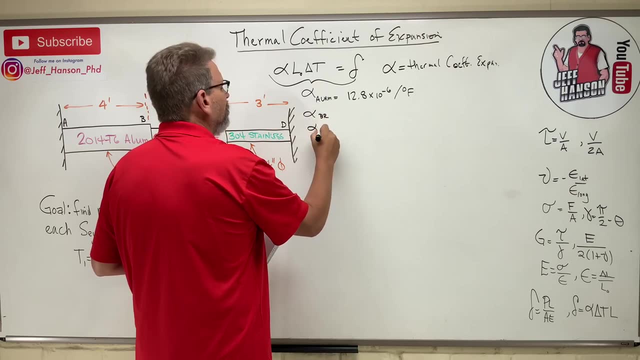 my book here and then I can put this book down. Let's look up the bronze and the stainless, and then we'll have all of these alphas over here, won't we? Okay, Br for bronze and St for stainless. Let's see what we got here. Bronze, where are you? bronze? There you are. 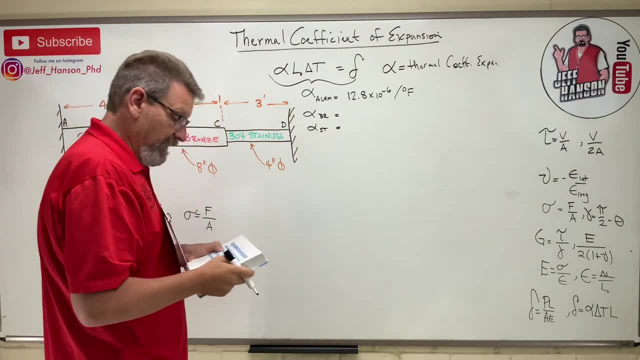 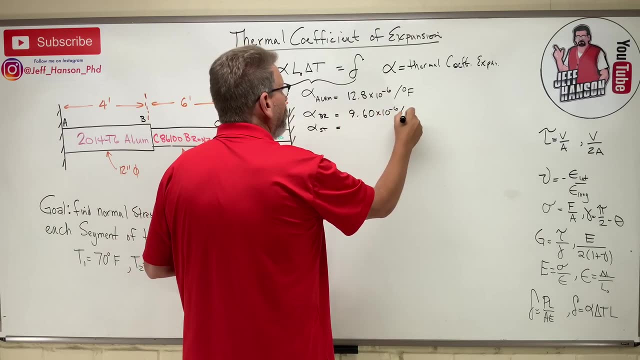 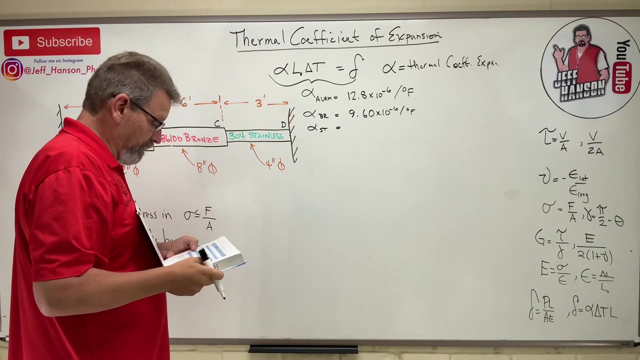 86 100 is what we're talking about here, and 86 100 is 9.60 times 10 to the minus 6 per degree Fahrenheit. and then stainless steel: 304 stainless. where is 304?? 304 stainless? 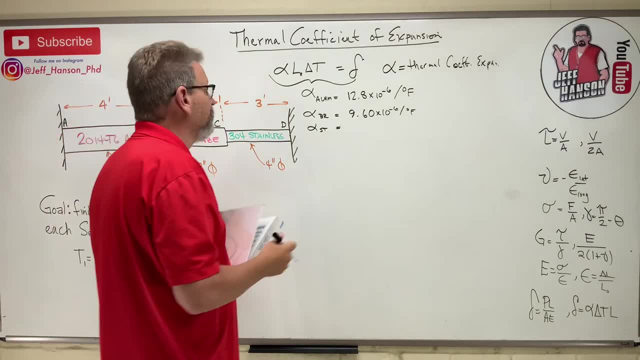 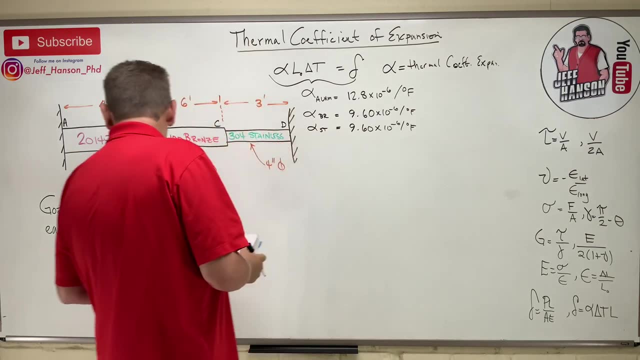 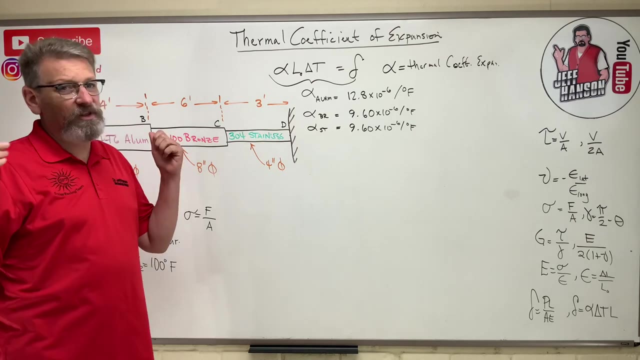 Stainless. there he is 9.60, it's the same, isn't it? 9.60 times 10, to the negative 6 per degree F. okay, So first thing we're going to do. this is kind of like the problem we did last time when we 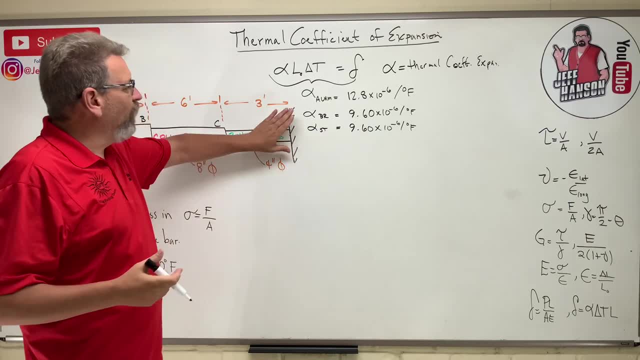 did the method of superposition. First thing we're going to do: we're going to take away this wall over here D and pretend it's not there, whoop. and we're going to let it grow. let it grow. 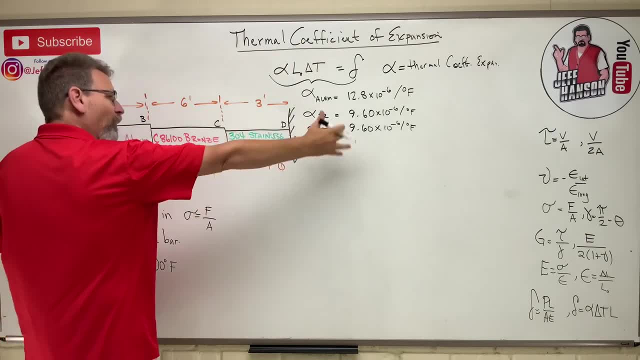 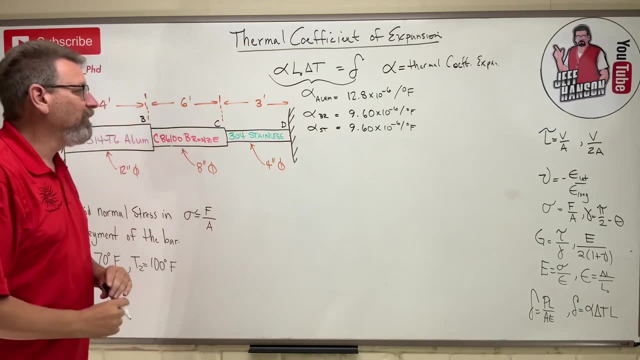 Oh, no, sorry. Okay, we're going to, We're going to let it grow without the wall there. Then we're going to put the wall back. and what's the wall going to do? It's going to push it back, right? Well, it's going to push. 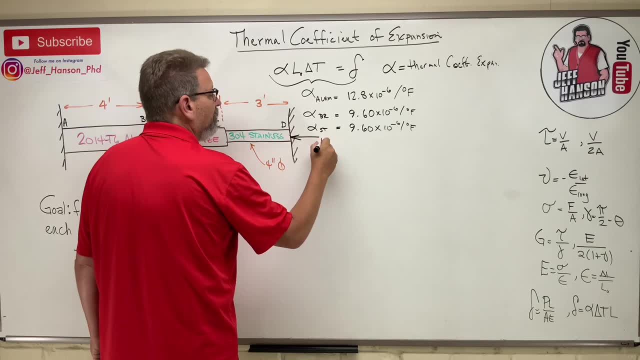 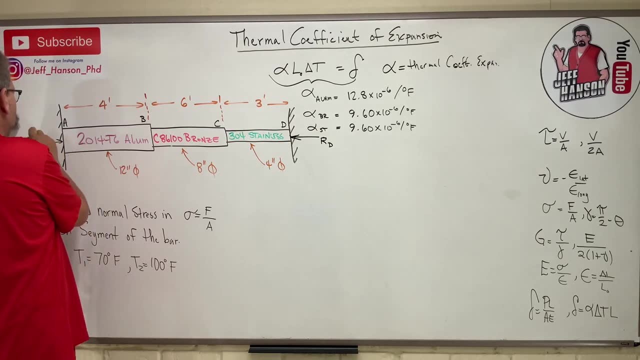 it back with some reaction force over here, some reaction at point D, okay, So, and this guy over here, of course I'll have a reaction at point A. So let's do this, Let's take that wall away. 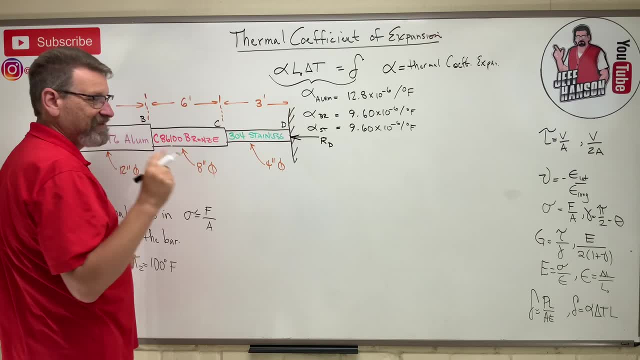 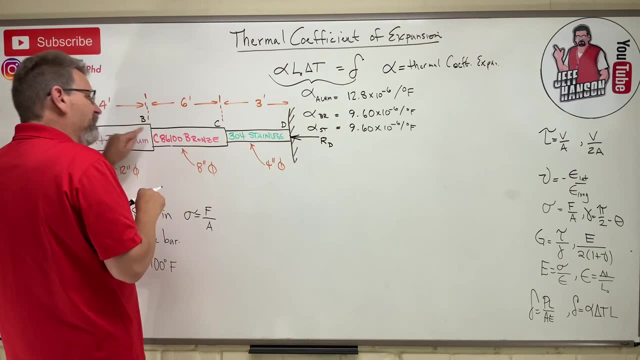 and let's let that grow and that grow and that grow and let's see how much it'll grow. So we're going to take this equation here and we're going to use find the delta for this one, the delta for that one and the delta for that one. So we're going to add them up, right? So 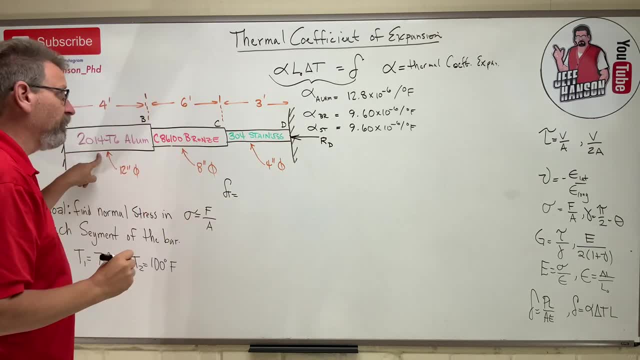 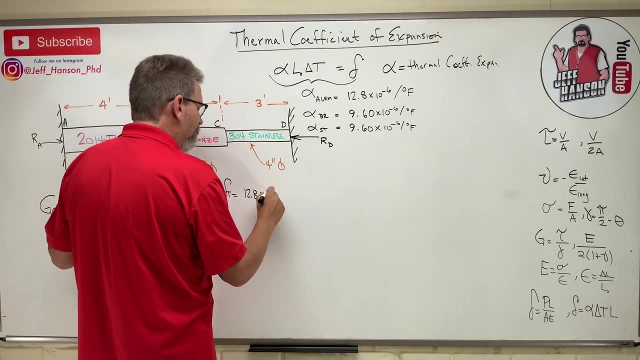 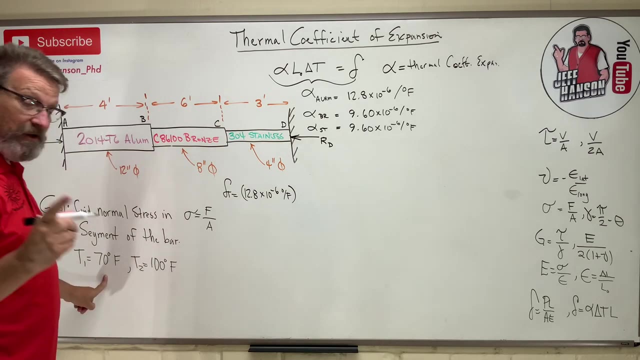 delta total is equal to all right. here comes the first one, the aluminum right. So the aluminum is 12.8 times 10 to the minus 6 per degree F times delta T, which is 30 degrees F. 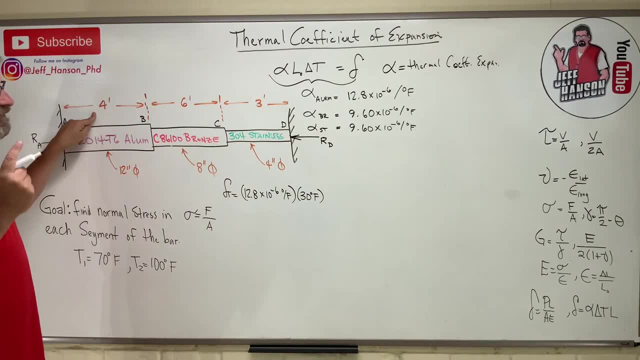 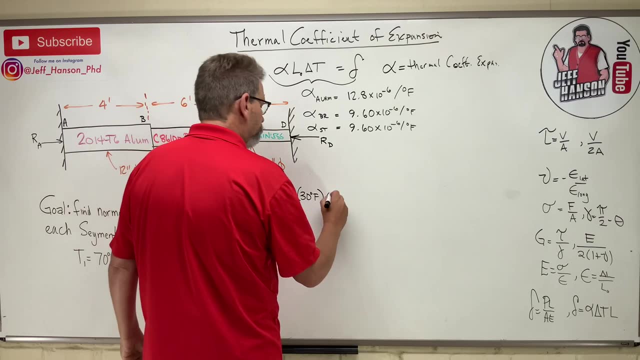 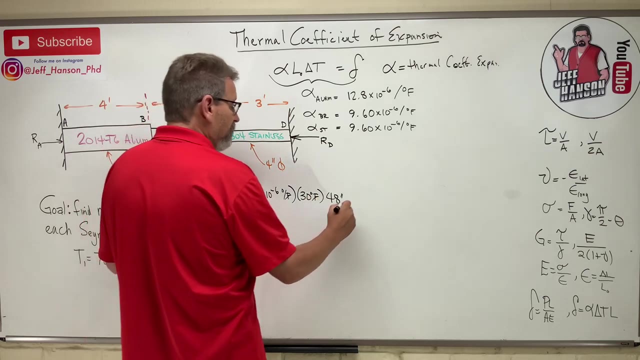 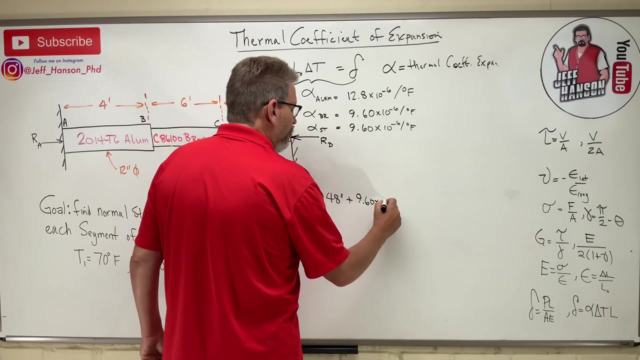 times L and this. this needs to be in inches. This is a little bitty number here We need to be in inches. How about 48 inches? That will give us our delta in inches, because that and that cancel out, don't they Plus? okay, let's do the next one, the bronze, 9.60 times 10 to the minus 6. 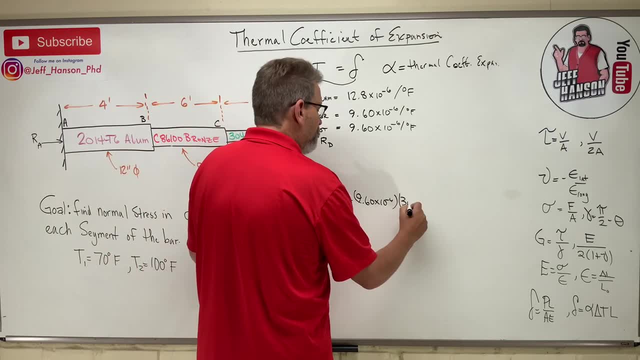 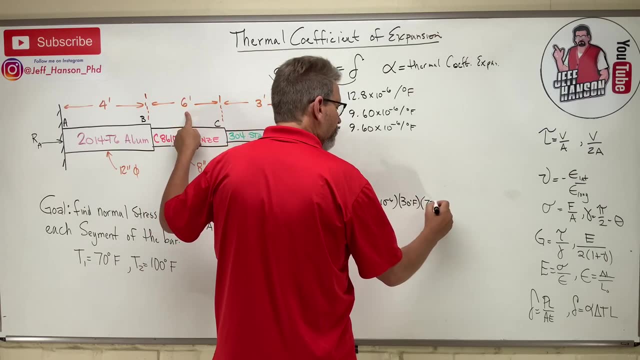 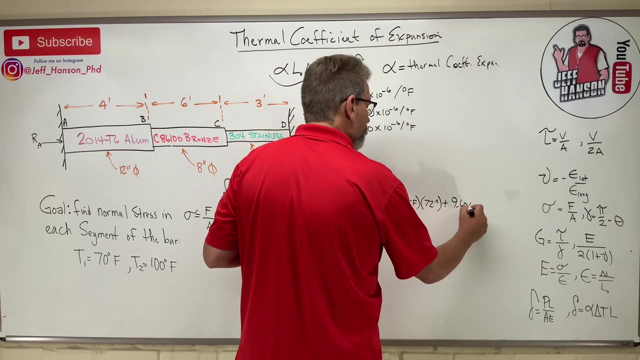 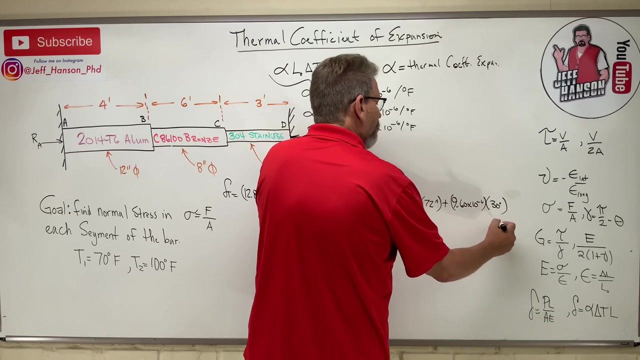 times same temperature change- Okay. and then times its length, which is 72 inches, isn't it Okay? and then one more plus 9.60 times 10 to the minus 6 times change in temperature, and then times its length of 36.. 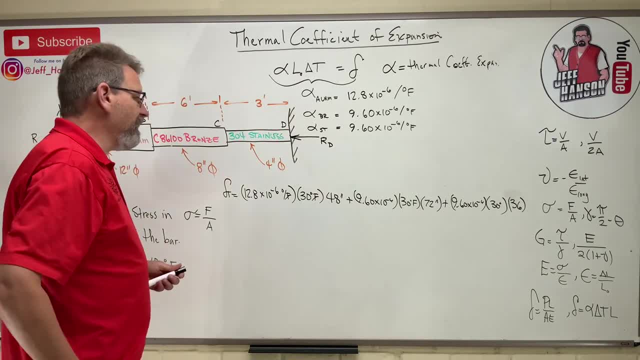 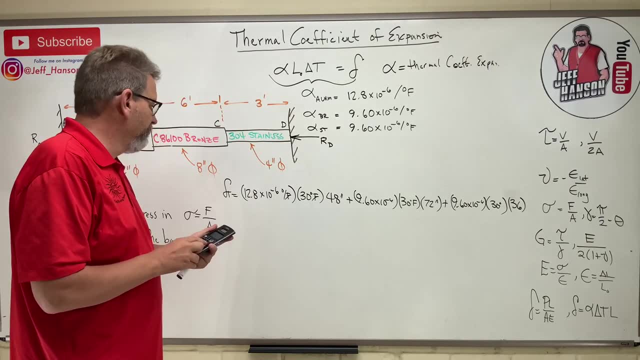 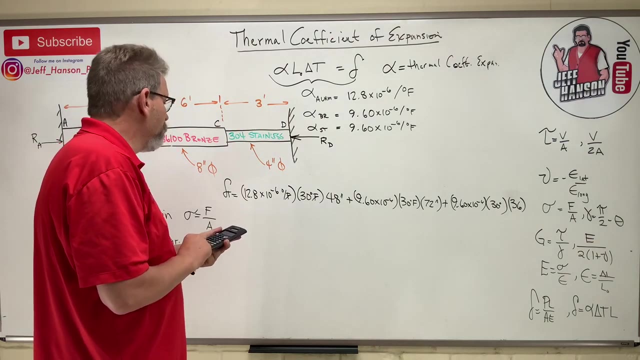 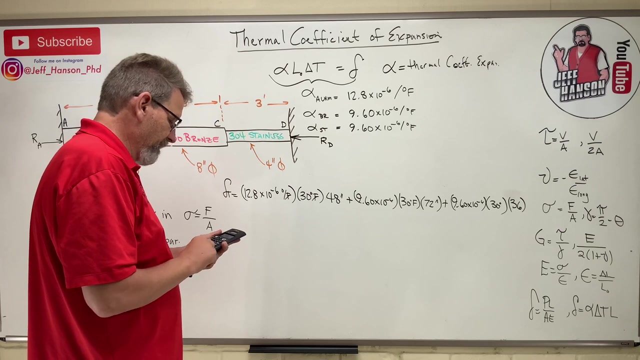 Okay, all right, it's time to get our calculator Now. we could factor a 30 out, but let's just do it. Here we go. Let's just do it, All right. so point 1, 2, 3, 4 zeros: 1, 2, 8 times 30 times 40, 48 equals. all right. so over here. 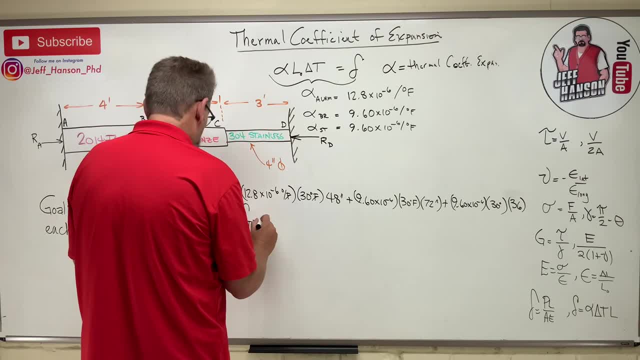 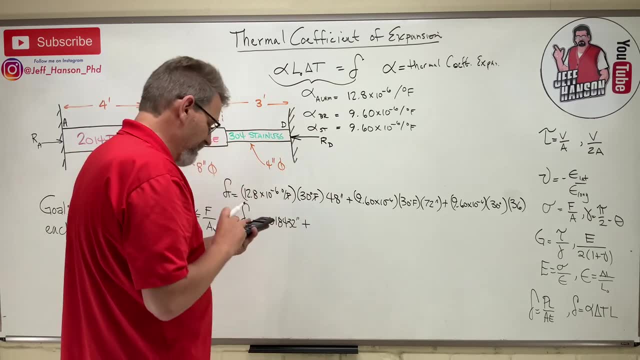 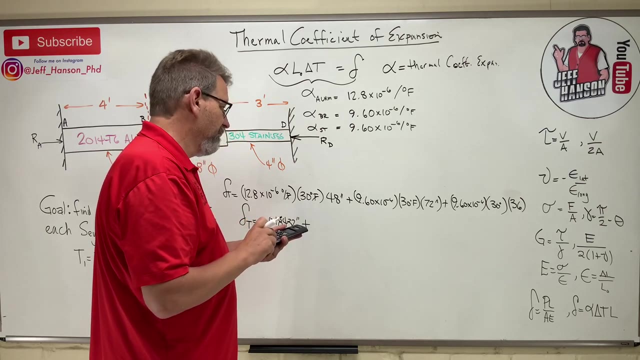 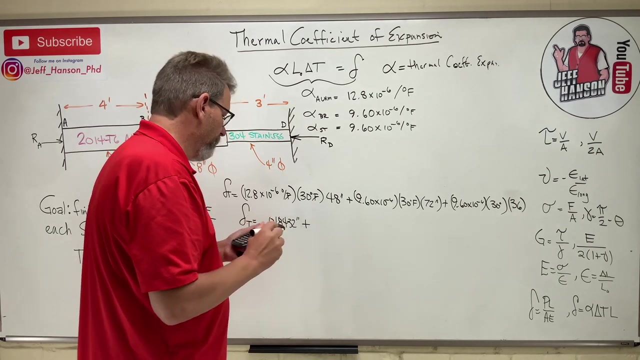 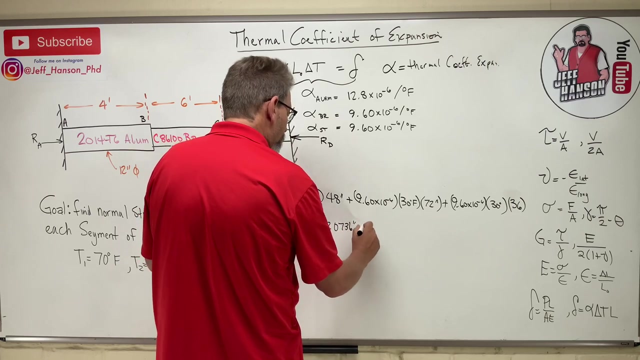 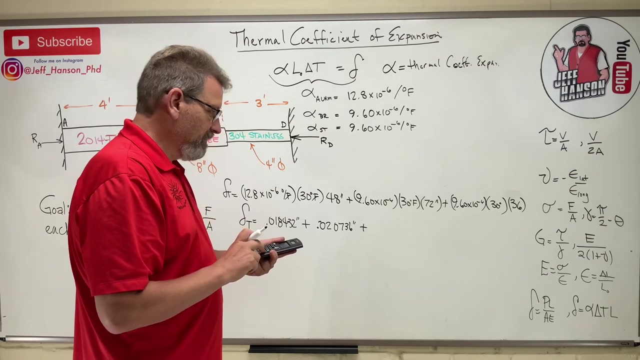 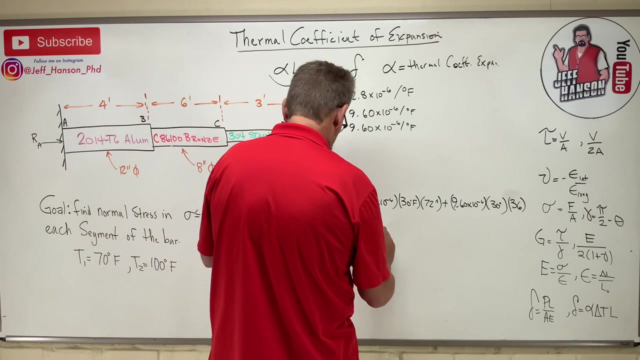 so delta total- it's equal to this guy- is 0.018432 inches, plus next 0.1234596 times 30 times 72 equals this guy 0.020736, and the last guy over there- 0.12345 zeros, and then a 9.60 times 30 times 36, that equals 0.010368 inches. 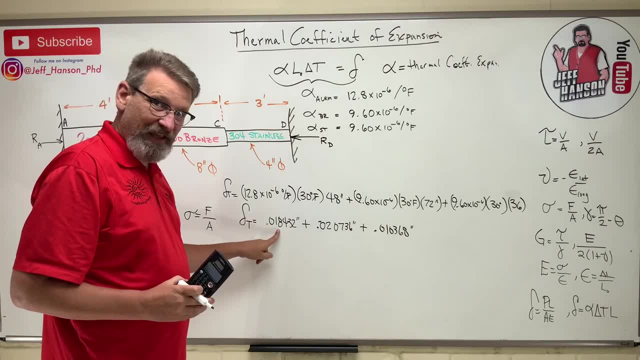 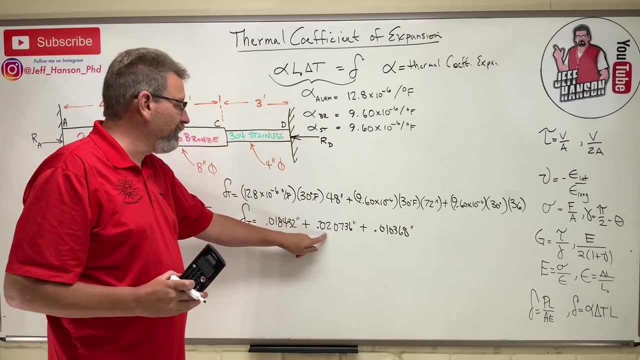 Okay, is that a lot? That's 18 thousandths of an inch right, That's about two and a half human hairs. thick. right, That's 20 thousandths. that's almost three human hairs and that's about a human hair. 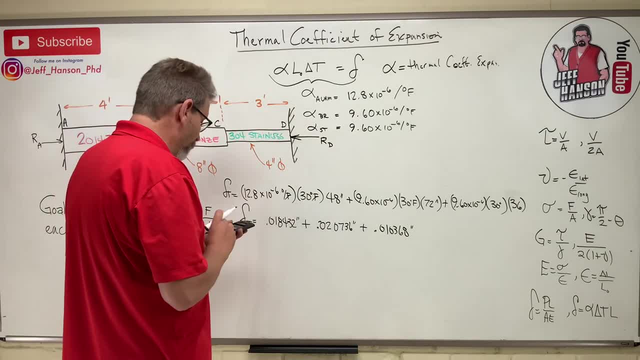 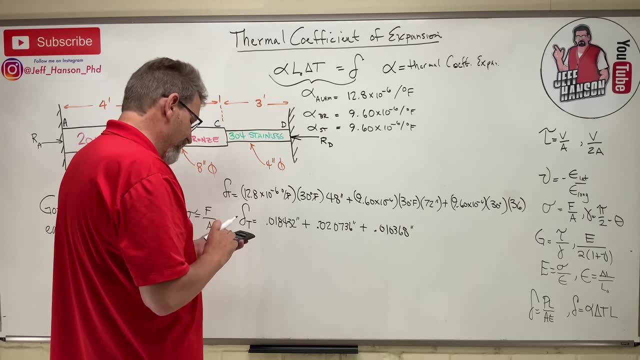 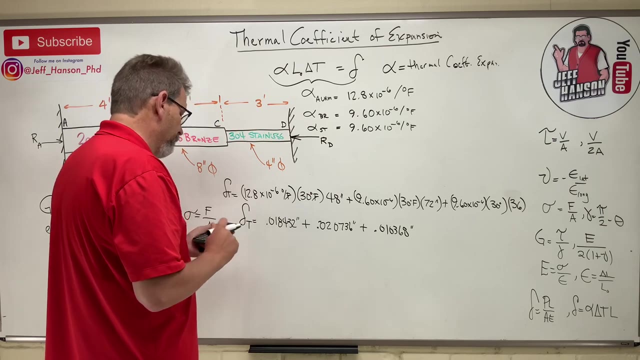 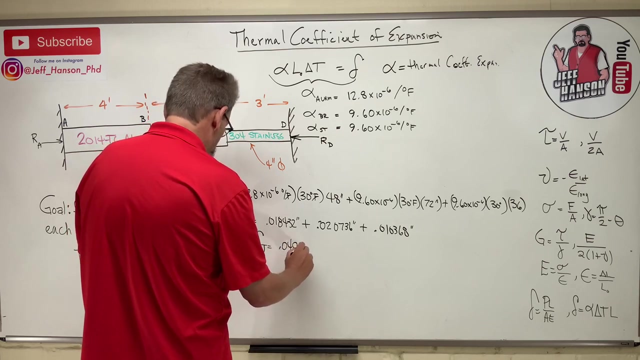 All right. so we're not a lot of growth, but you know some, Okay. so that number over there plus 0.020736 plus 0.018432 equals all right. so delta total is equal to 0.049536 inches Again. 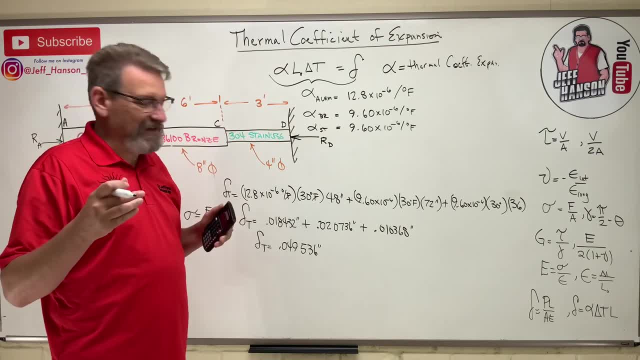 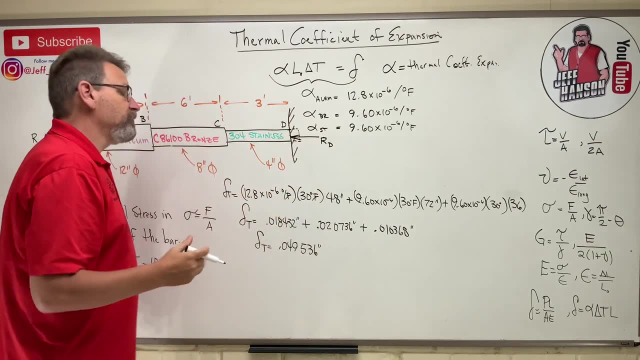 leave lots of decimals and then we'll round at the end, okay, So without the wall there, this whole thing is over here now. okay, So we've got to push it back. Now what are we going to push it with? A reaction force. So? 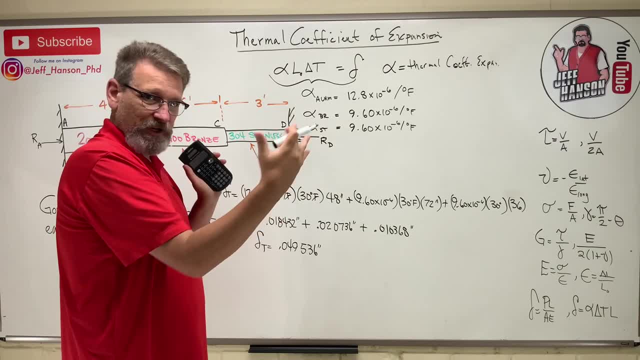 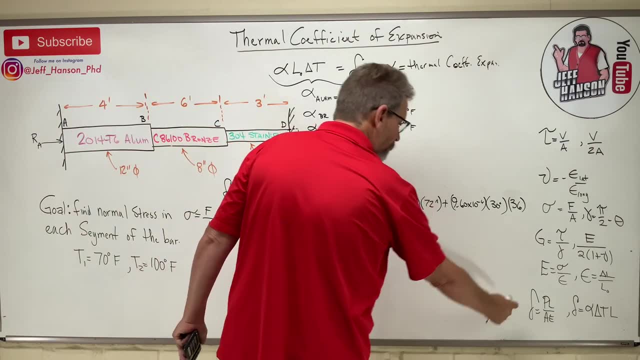 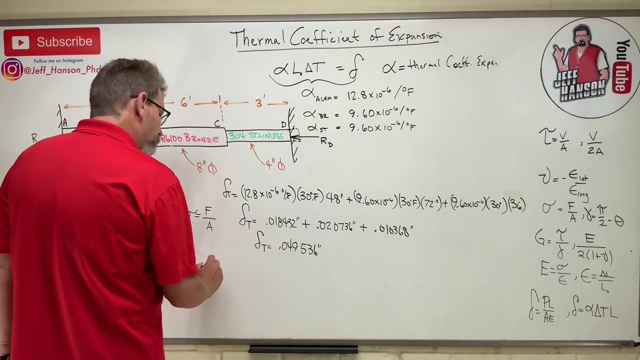 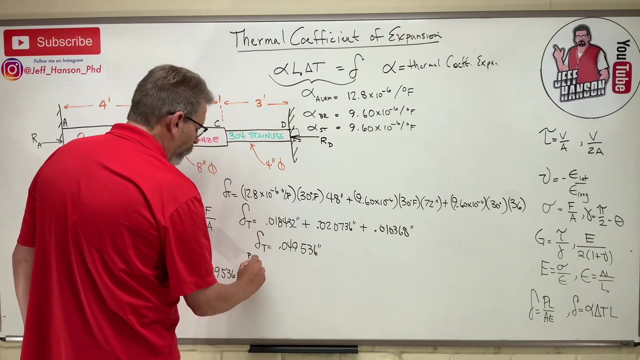 now we're going to have an axial elongation, really an axial shortage due to a force. Hmm, what equation would that be? Oh, that one, right there, right, So delta: total: 0.049536, right, That is our total. delta is equal to what? Well, pl over A E for section one. 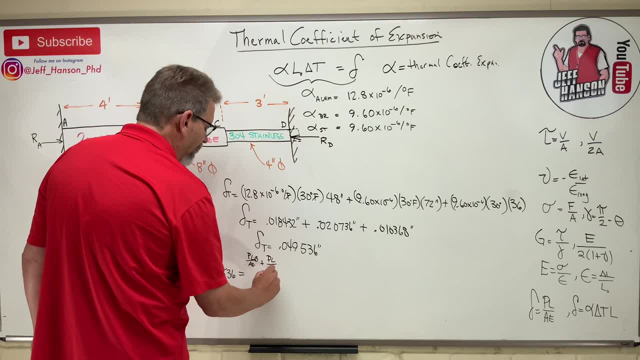 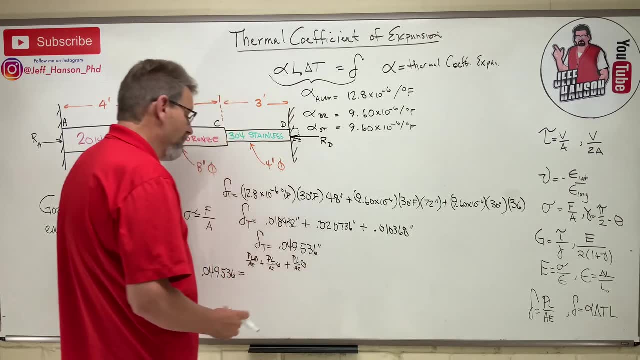 plus pl over A E for section two, plus pl over A E for section three. right, So this, and who's what's p? P is this rate, Yeah Well, okay. so what we want to be doing now we are, So we want to. element. so you go all the way right across from here, all right. So what we want to do here is- and I think that a few times you should know, you know bu lok Е is equal to, and not just longer. 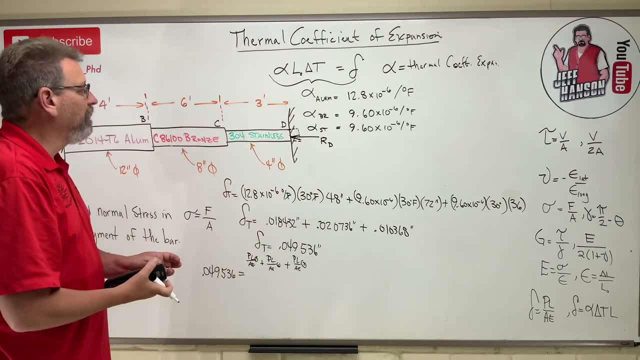 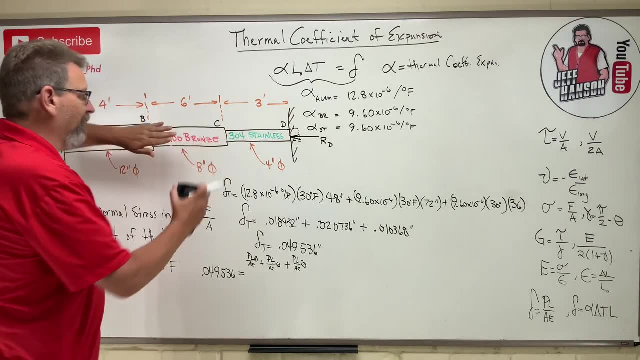 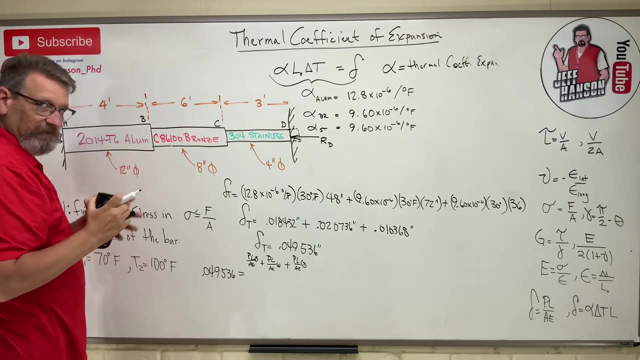 P? is this reaction force right here? Do you agree that, whatever that reaction force is, that's the force in this member, in that right? Cover it up, right, That's Rd. Cover it up, that's Rd. Cover it up, that's Rd. right, And what else do we know? Rd is going to be equal to Ra. 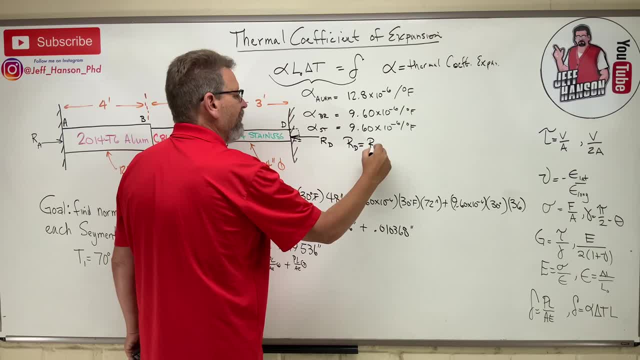 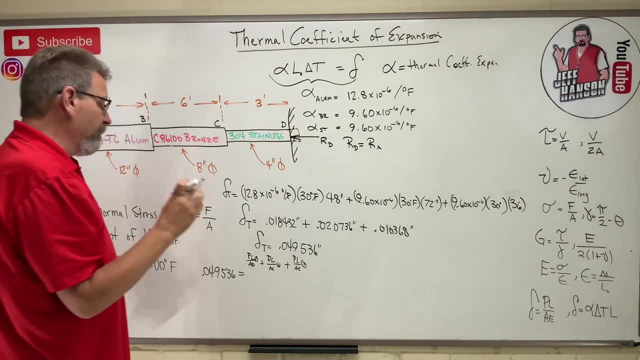 right, I know that The reaction at D is going to be equal to the reaction at A, because there are no other applied forces on this problem. right, All right. so all we need to do is these Pl over Aes for each one of those, And so you know, it's got to compress that much And who's 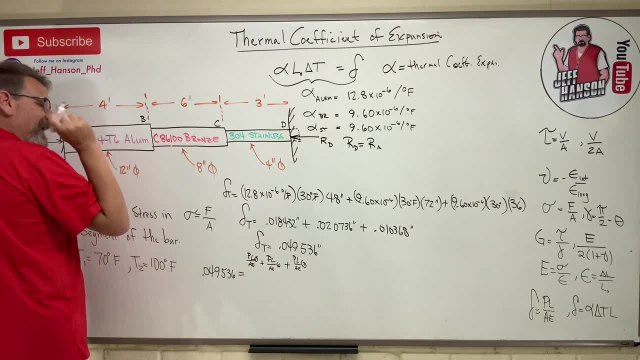 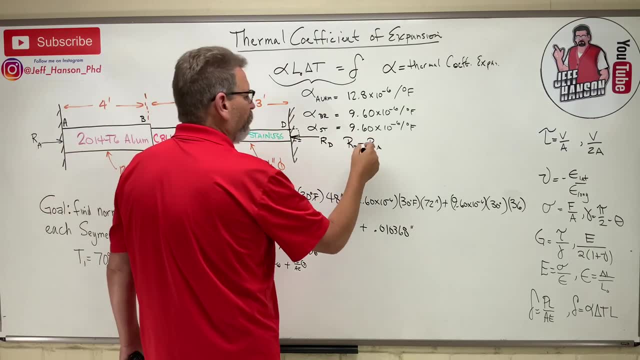 going to compress. Well, he's going to compress a little. he'll compress a little, and that one will compress a little. okay, So let's write our Pl over Aes for all of these. Since Ra equals Rd, let's just call that F. okay, That's just the force, the reaction force I'm just going to call. 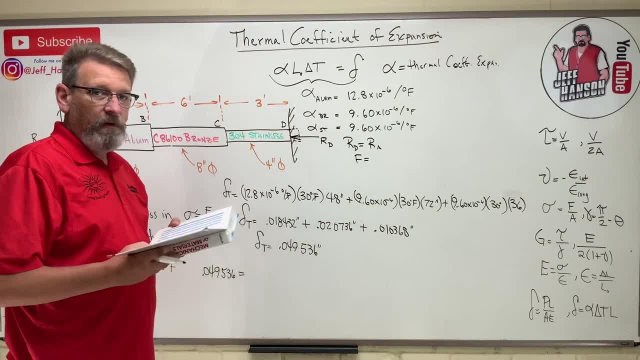 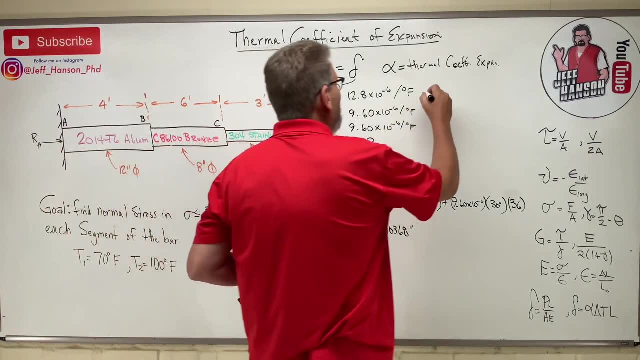 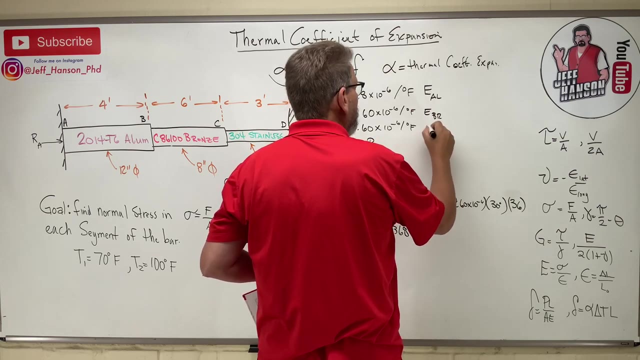 it F. okay, So here we go. All right, I'm going to need my table one more time because I am going to need Pl over Ae. I need E, don't I? So I need E for each one of these materials. So E aluminum, E bronze and E steel. 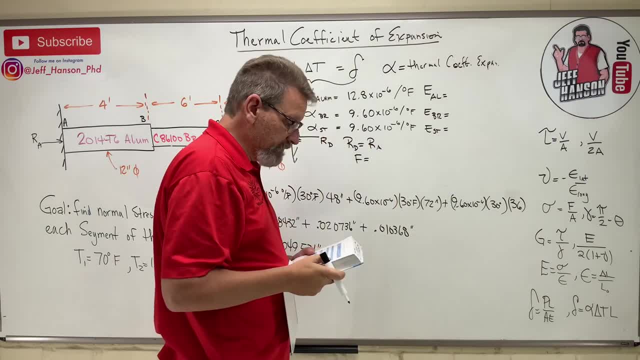 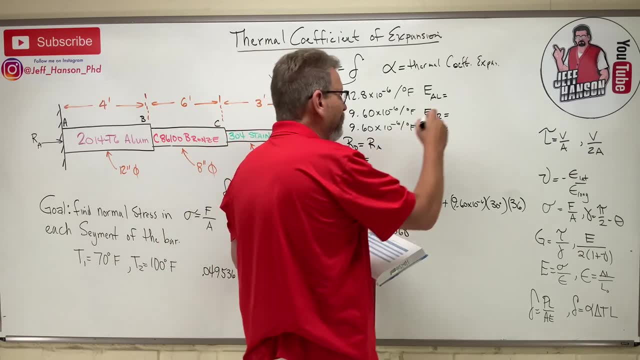 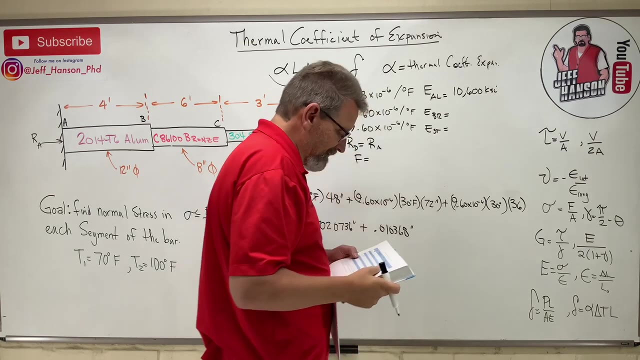 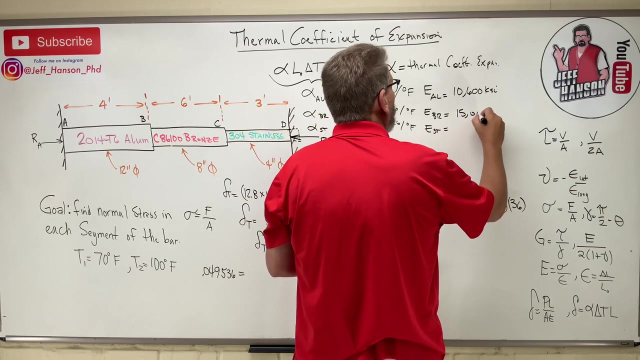 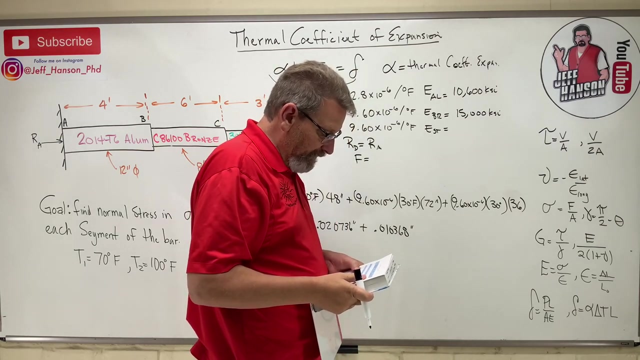 I need those, don't I? I need that. All right, modulus elasticity for 2014: T6, 10.6 times 10 to the 3,, which is 10,600.. KSI Bronze: bronze 86100 is 15 times 10 to the 3, KSI- okay, And then finally, stainless steel: 304. 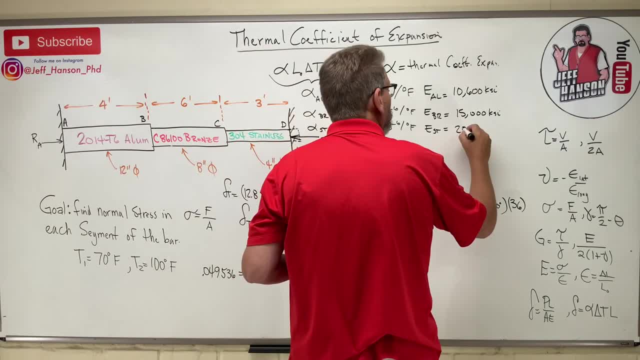 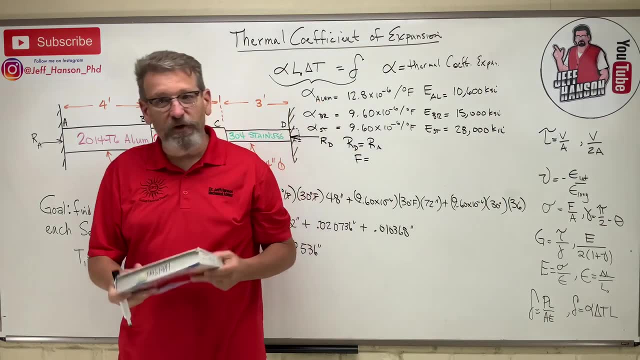 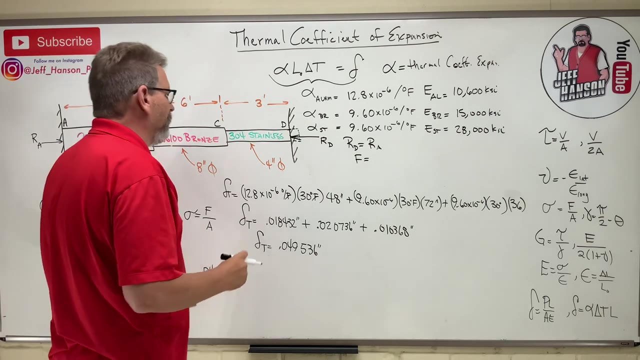 is 28 times 10 to the 3, KSI. okay, So there's my values out of the book. I don't think I'll need the book anymore, but I will need my calculator. All right, here we go. Pl over Ae for each one. Let's do. we'll do aluminum, bronze and the 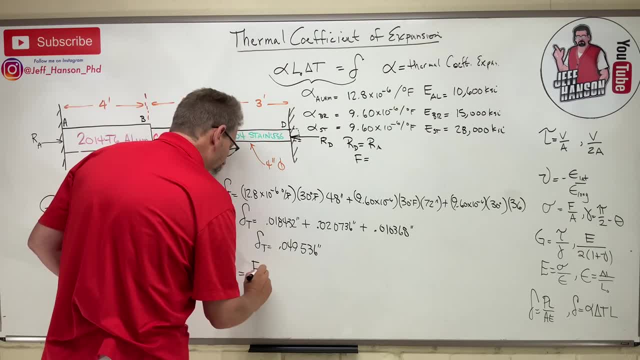 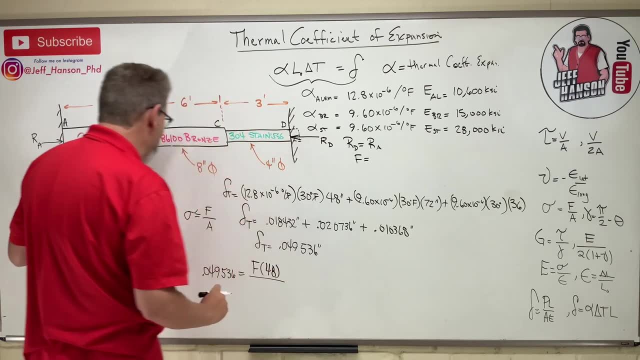 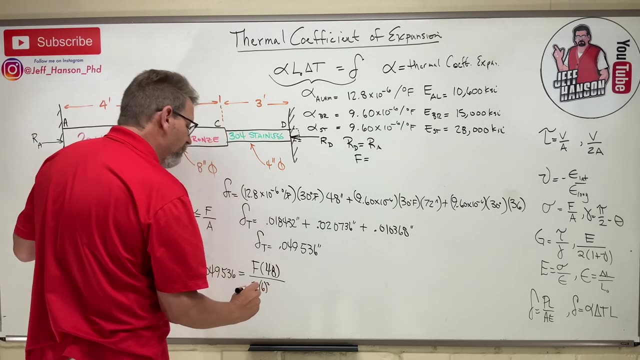 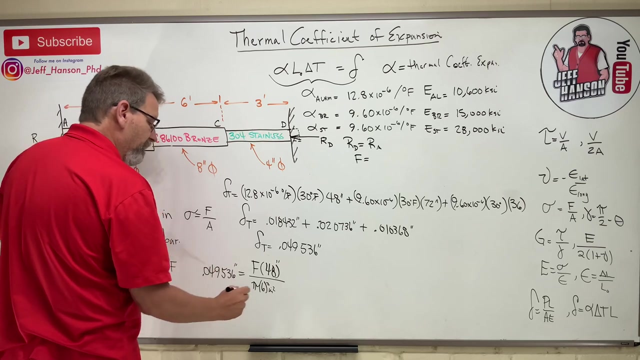 stainless. So for the aluminum, the force is F, The length is 48 over A, The diameter is 12 inches, so that's pi times 6 squared. right, And this was in inches. This is in inches squared. This is in inches over here. And then the E is in what is E in KSI. okay, So that's going to be. 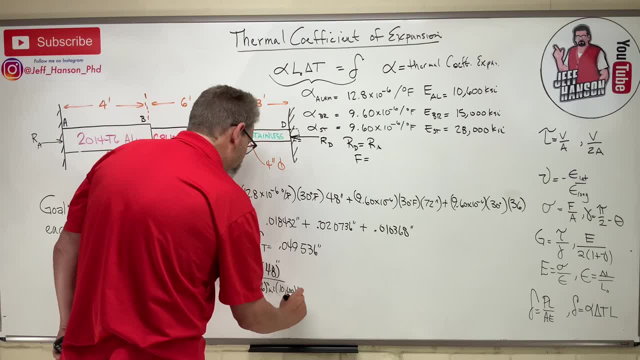 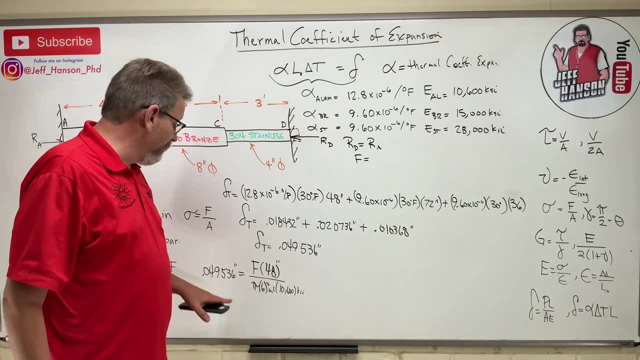 10,600 KSI. So that tells me, because KSI is kips per square inch, right, The square inches. cancel out, the inches and the inches cancel out and just leave me with kips, right, So F. 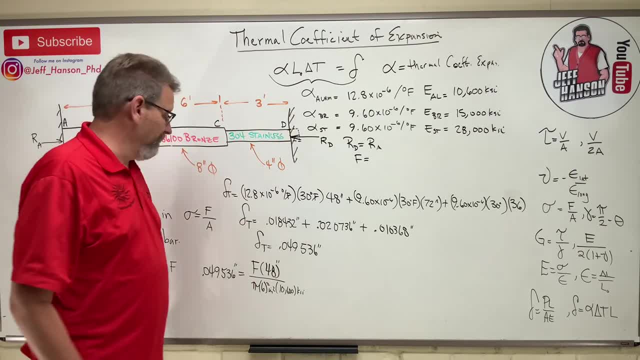 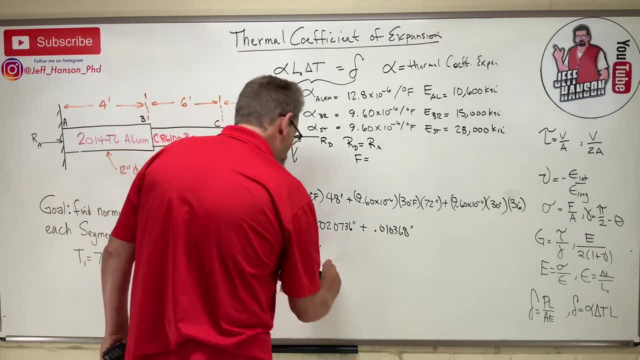 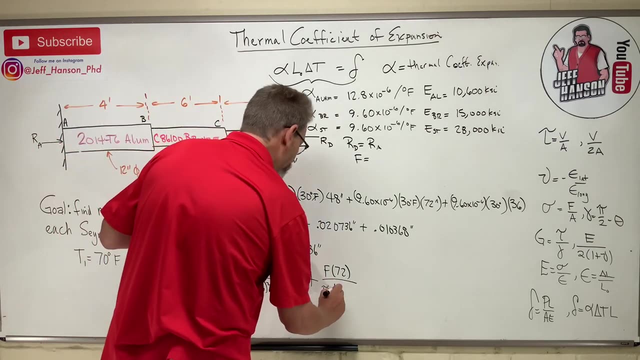 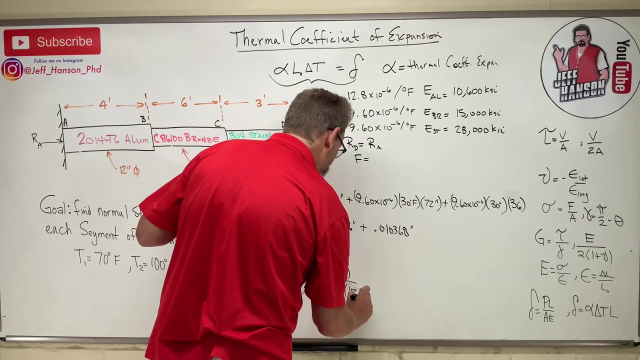 when I find F here, it's going to be in kips, isn't it Okay? so plus okay. here comes Pl over Ae for the bronze. okay, And that would be F times 72 divided by pi times. what's the radius there? Four squared times E for bronze: 15,000, okay, Plus one more. 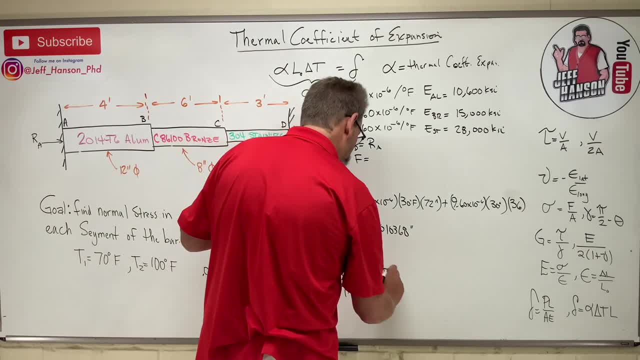 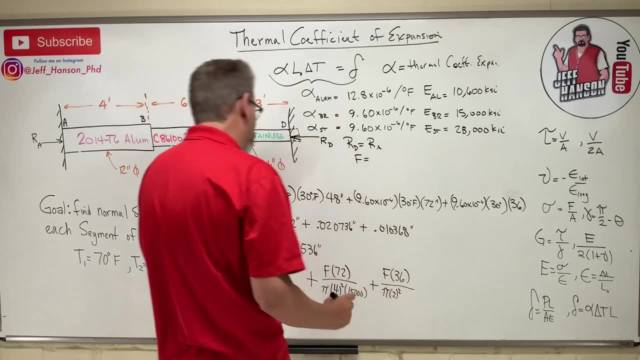 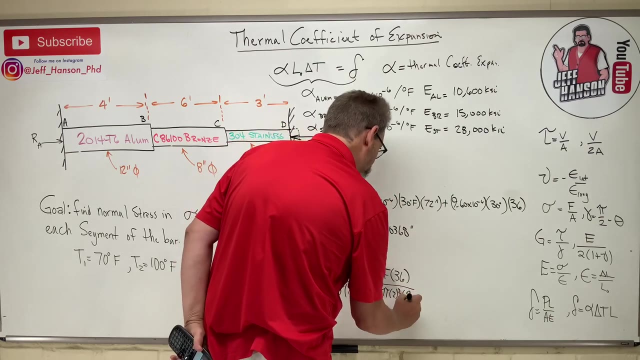 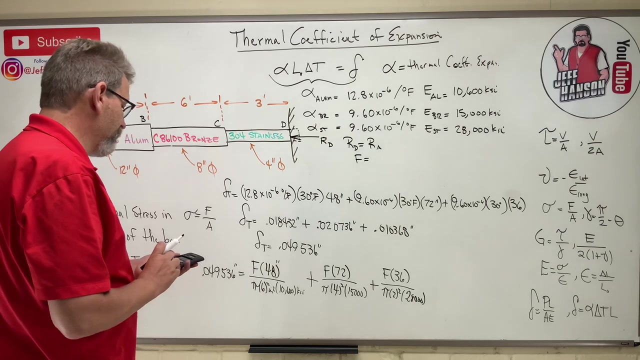 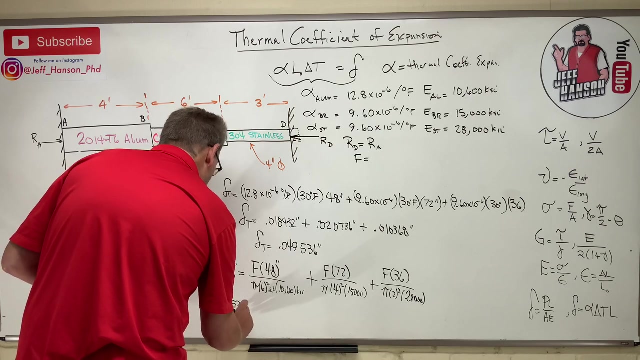 Pl over Ae for the stainless is going to be F times 36, divided by pi times two squared- because that's a four inch radius diameter, rather sorry- times 28,000, okay. So let's do a little. let's do a little calculating, okay. So this is 0.049536 equals. 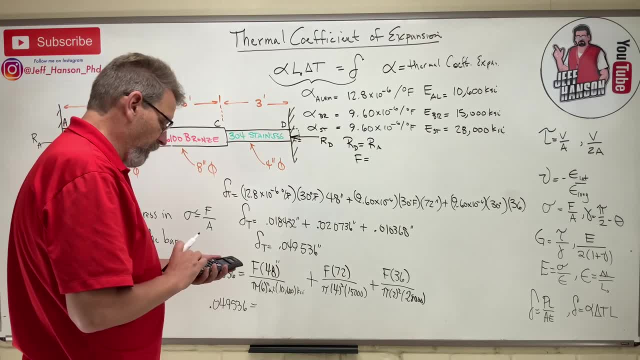 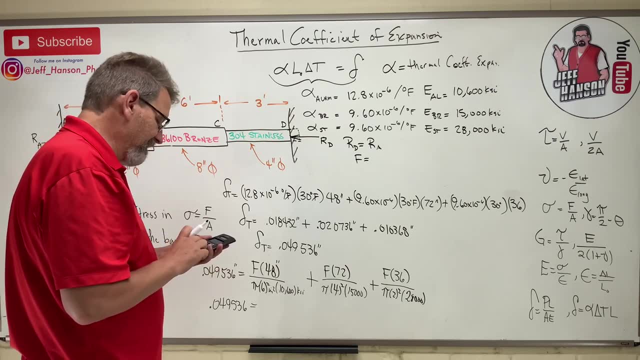 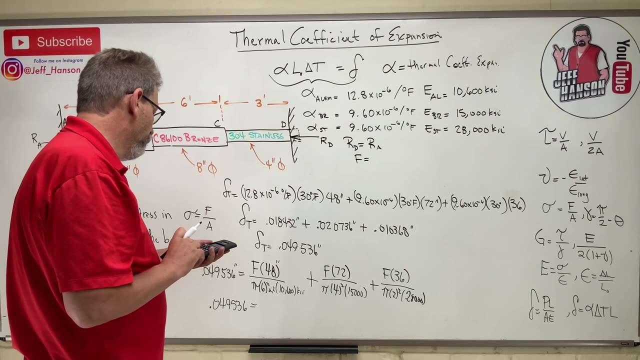 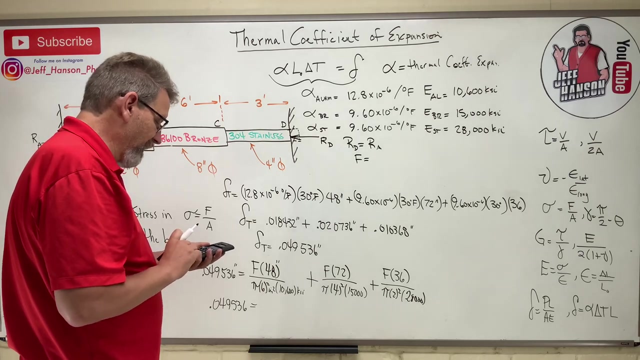 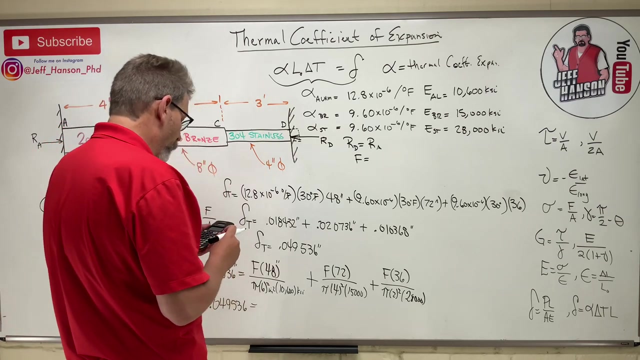 all right, how much is this 48,? oh, unclear. Come on calculator, wake up. All right, 48 divided by pi equals: um yeah, divided by pi divided by six squared equals. divided by 10,600 is one, two, three, four zeros. 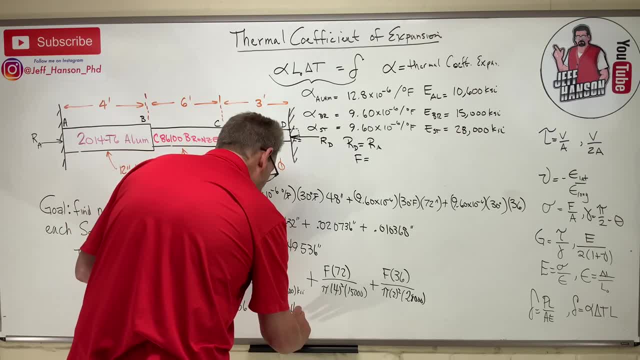 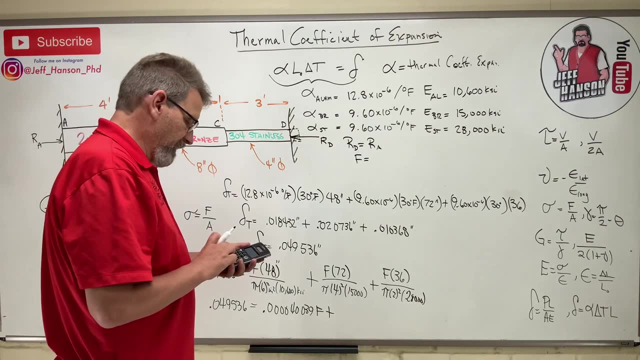 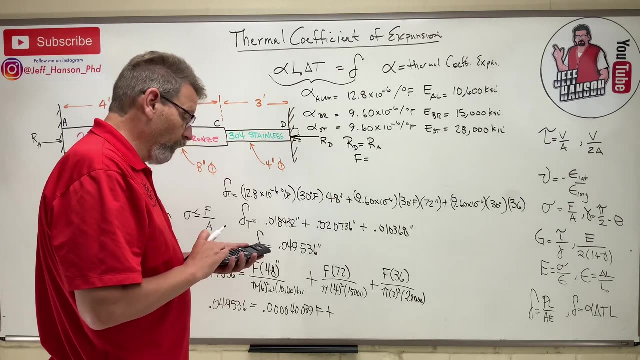 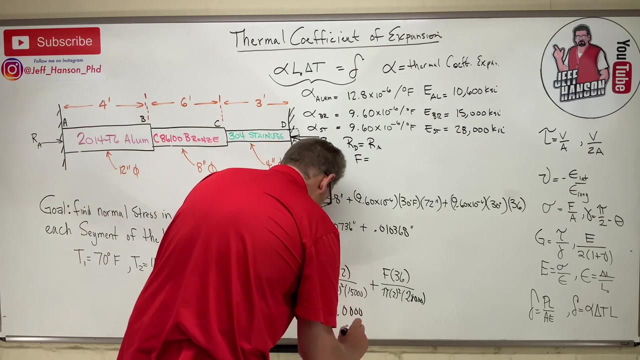 And then a 439, 439 F plus 72 divided by pi equals divided by four, squared equals divided by 15,000 equals one, two, three, four zeros. One, two, three, four, and then a nine five, four, nine three F. 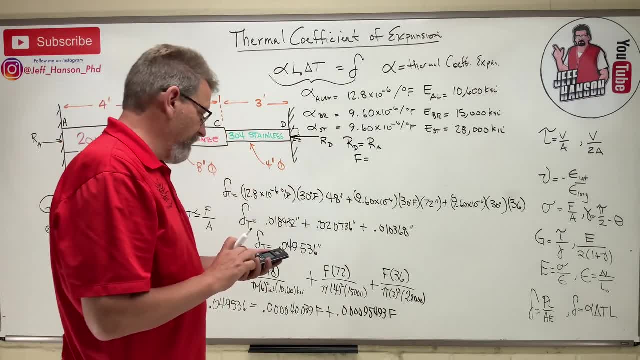 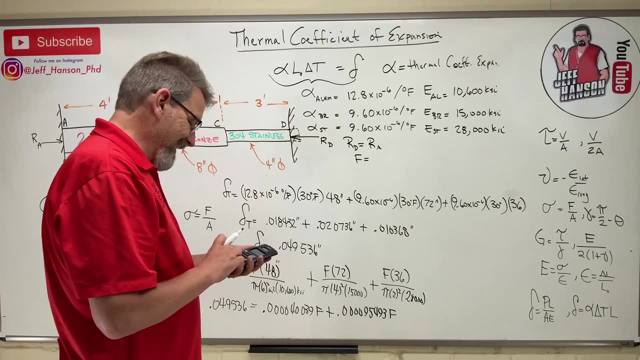 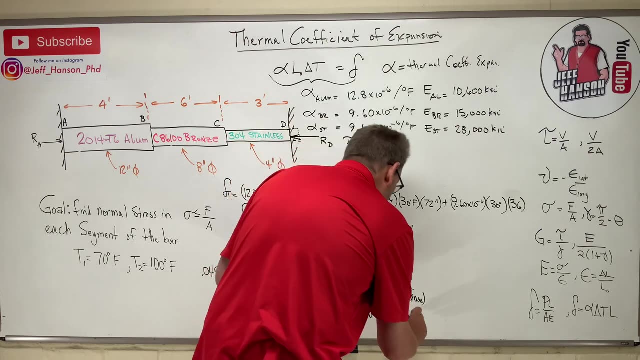 One more: 36 divided by pi: equals. divided by four: equals. divided by 28,000: equals. okay, plus three zeros: one, two, three zeros: 102,. three, one, four F. okay, So let's add all our Fs together. 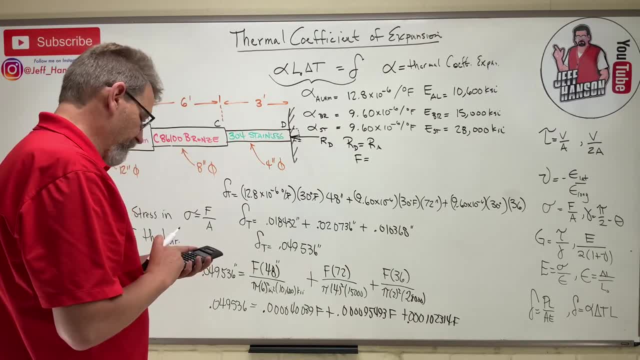 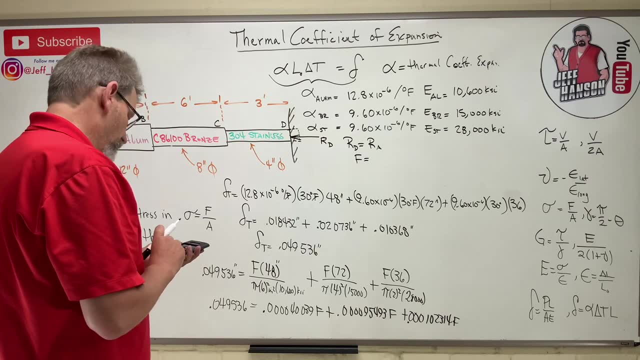 So that one plus point one, two, three, four, nine, five, four, nine, three, nine, five, four, nine, three plus point one, two, three, four, four, zero, zero, three, nine equals, okay. 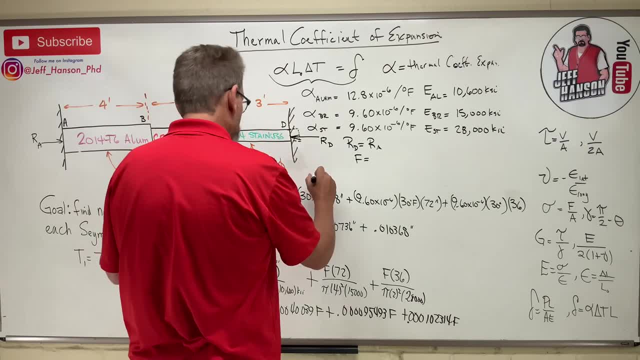 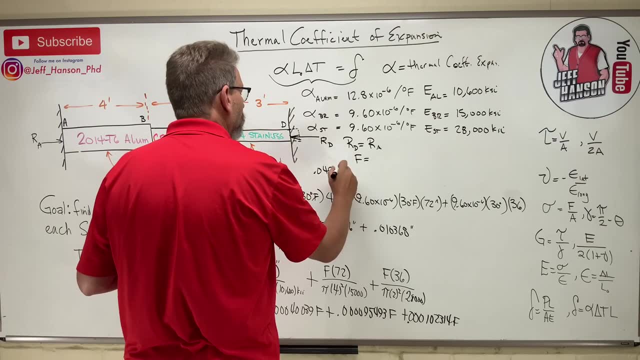 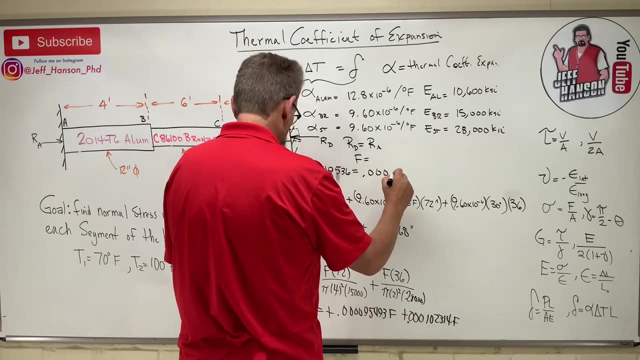 So that whole thing equals this: um point zero, four, nine, not uh, five, three, six. Oh no, Is equal to point zero. zero zero two, three, seven, eight, four, six, F. 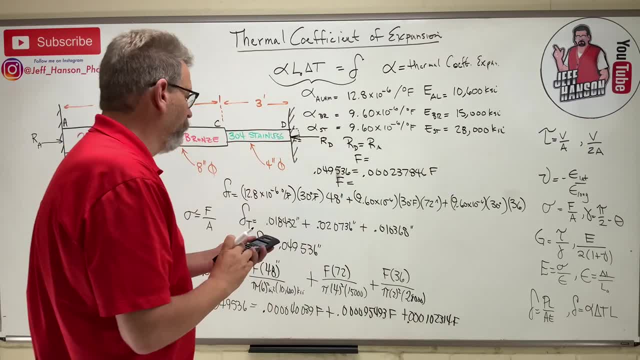 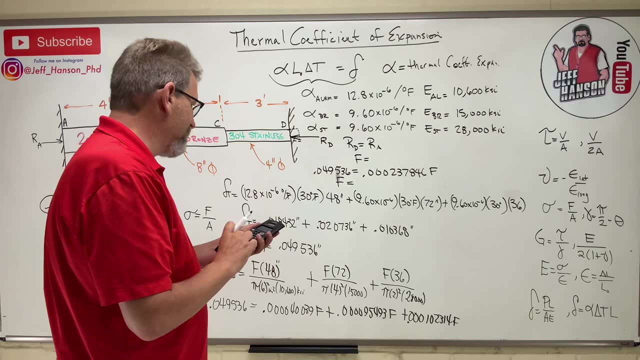 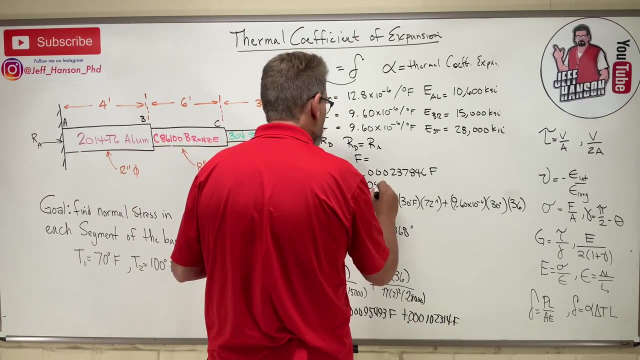 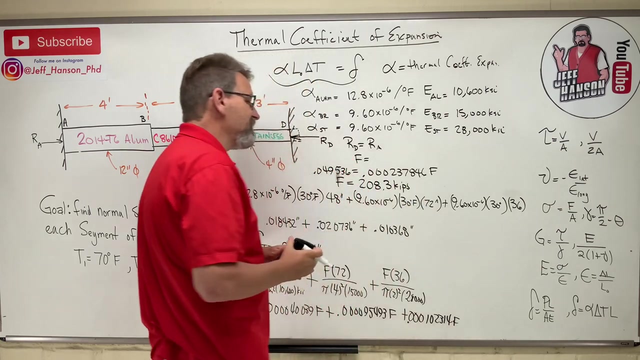 So F- and this is going to be in kips right- Is equal to. here we go. point zero, four, nine, five, three, six, divided by answer equals 208, point three: kips. Now you see why I carry so many decimals. 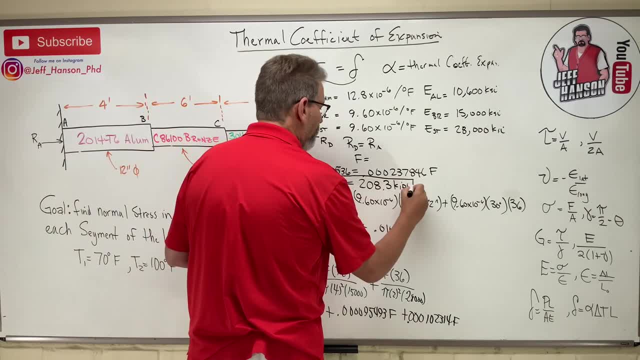 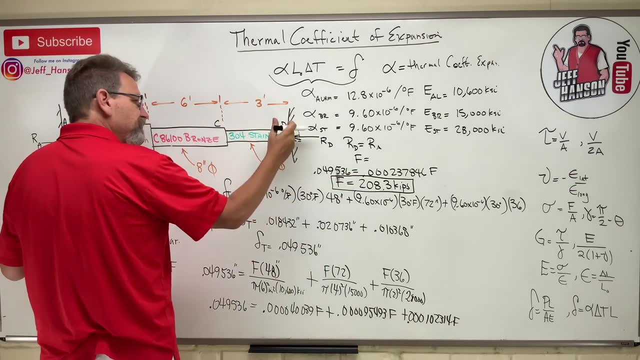 because when we do that division, uh, they kind of matter, don't they? Okay, So there's the force, that reaction forces. that thing grew. it generated 208 kips, which is a thousand pounds. right, That's about a kilopound. 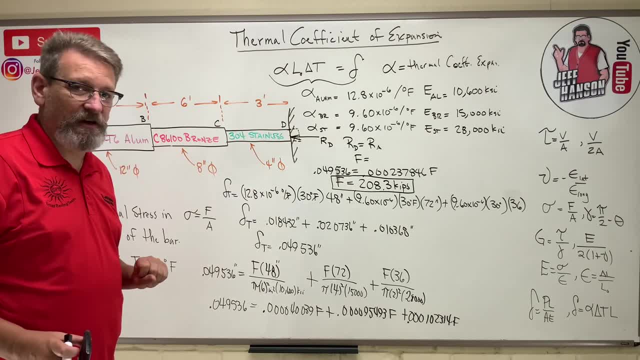 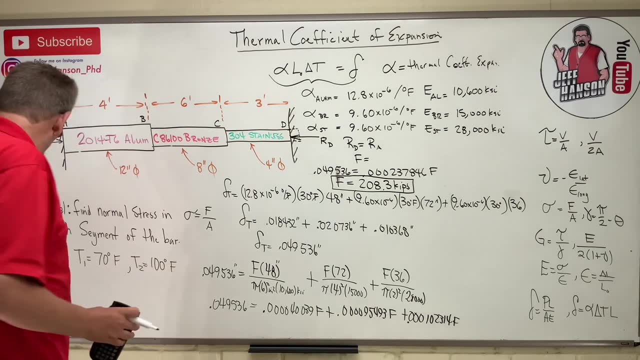 So now we know how this, this thing, uh, from the the thermal grew and caused the force. So how are we going to? the original question was: what is the normal stress in each one? All right, so let's make us a little room here. 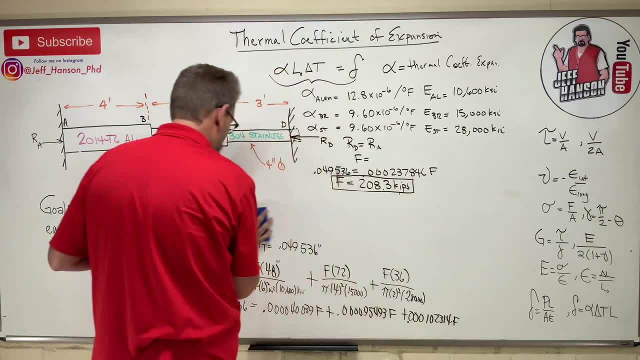 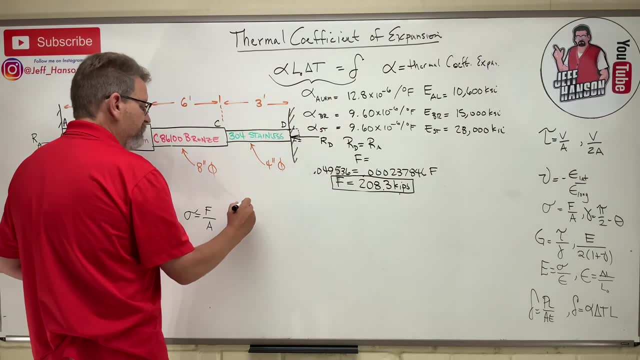 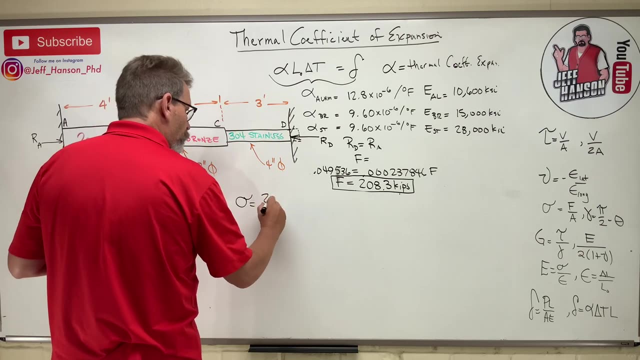 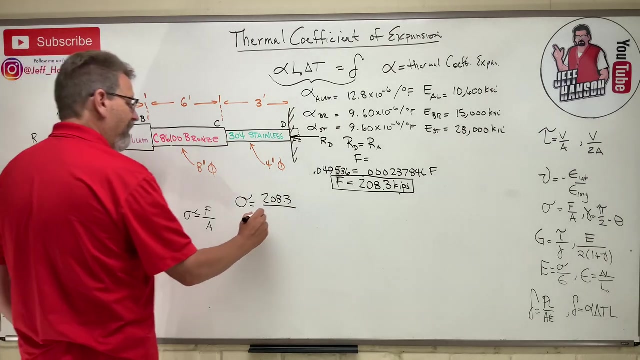 for our last little thing here. Okay, So here we go. Sigma for the aluminum right. The aluminum is F 208.3 divided by 208.3 divided by the area right, Which is going to be pi times six squared. 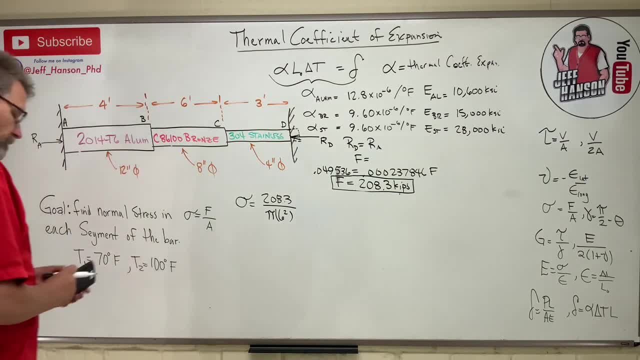 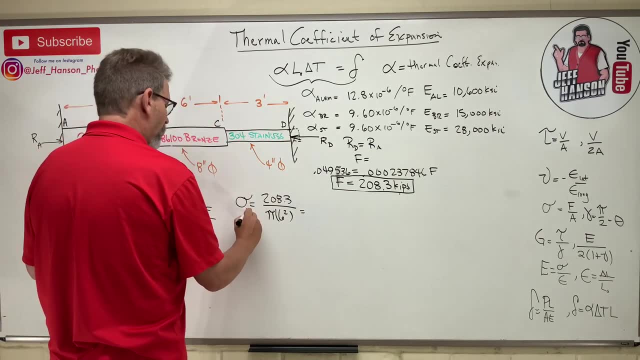 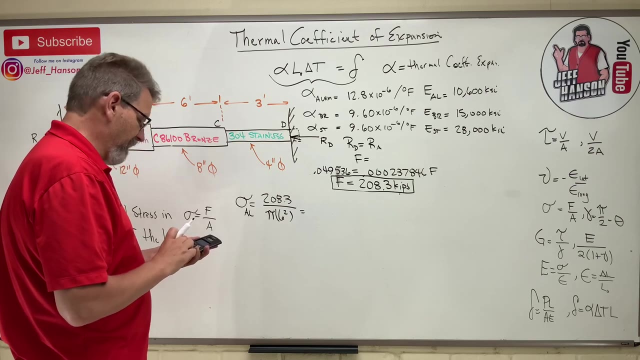 Okay, That's it, And let's. and that's going to be kips per inch squares, That's going to be KSI. So sigma aluminum is equal to 208 divided by pi: equals. divided by six squared, equals 1.84.. 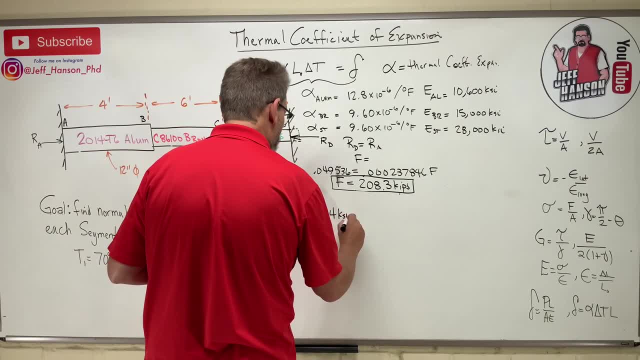 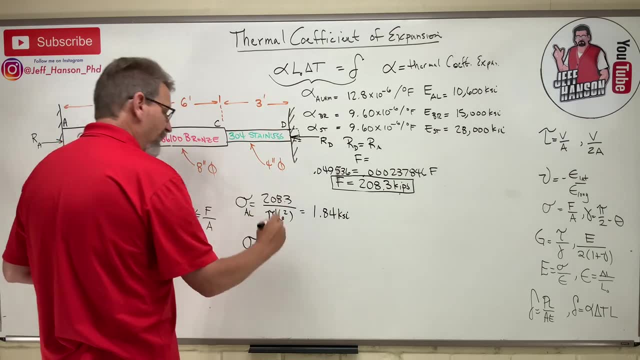 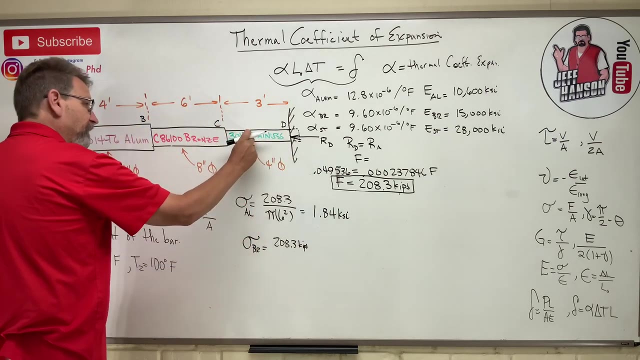 Okay, There's the normal stress in the aluminum. The normal stress in the bronze is going to be same over there, 208.3 kips, because that force is the same in here and there and there The force in those is the same. 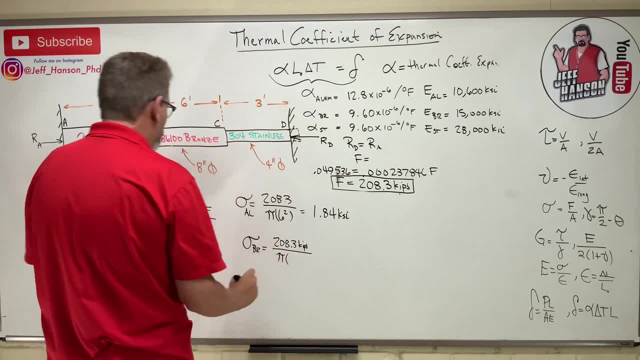 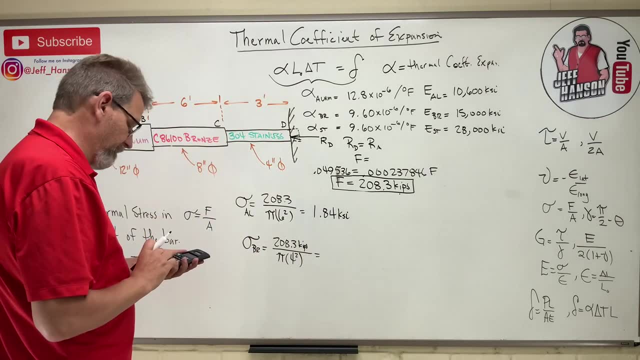 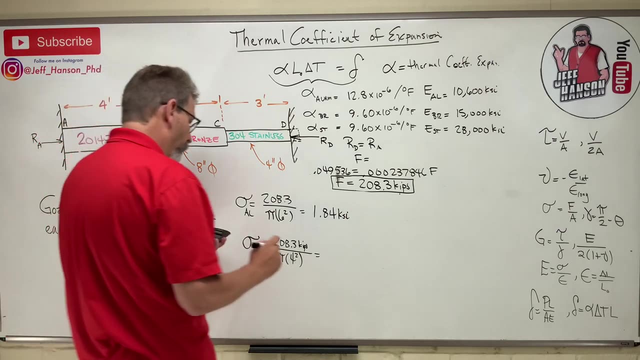 The area not the same. Pi times half of that's four. four squared equals. that's going to be in KSI. So 208.3, divided by pi equals. divided by 16 equals 4.14.. And we expected to get a higher number, right. 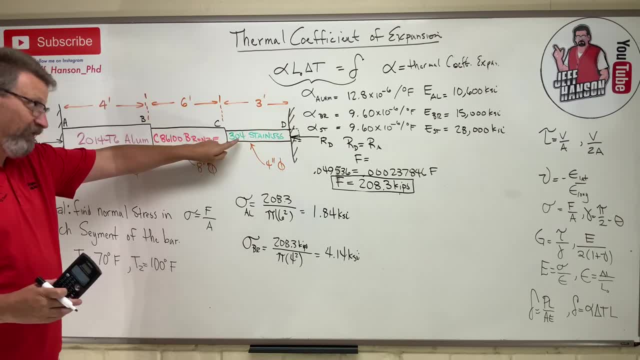 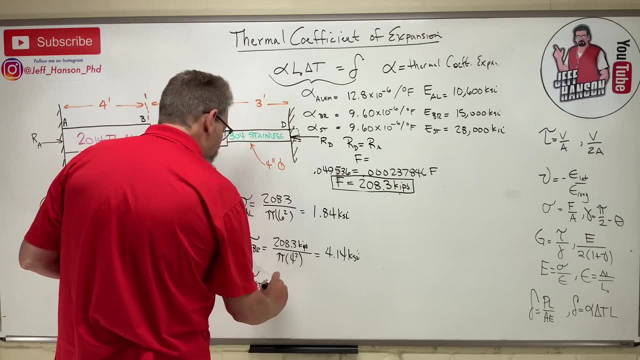 Because, guess what? The force is the same, but the area is going down. This guy should be even higher. Okay, So the stress, the normal stress in the stainless steel, is 208.3 kips divided by pi equals. divided by pi equals. 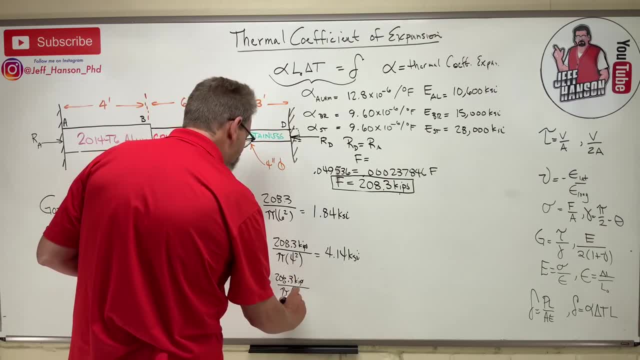 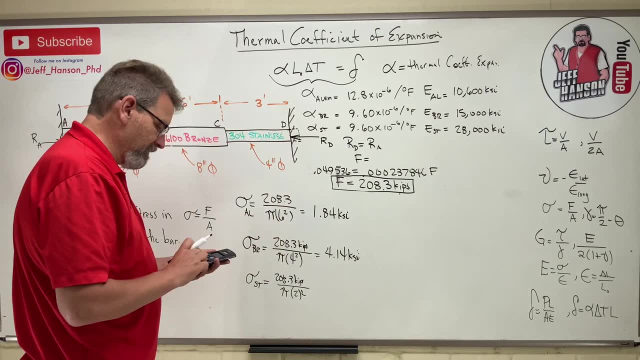 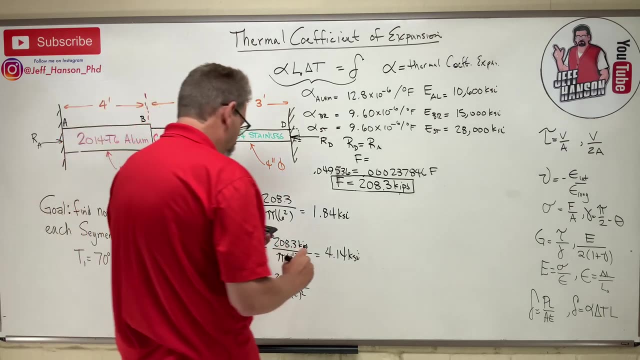 divided by 16 equals 4.14.. Okay, So the stress, the normal stress in the stainless steel is 208.3 kips divided by pi times three squared times 2 squared right. So 208.3 divided by pi equals. divided by 4 equals 16.58..